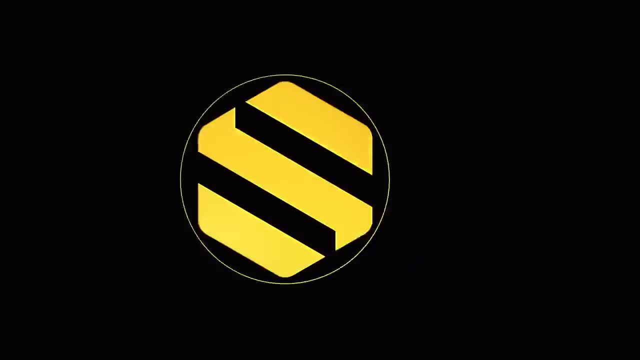 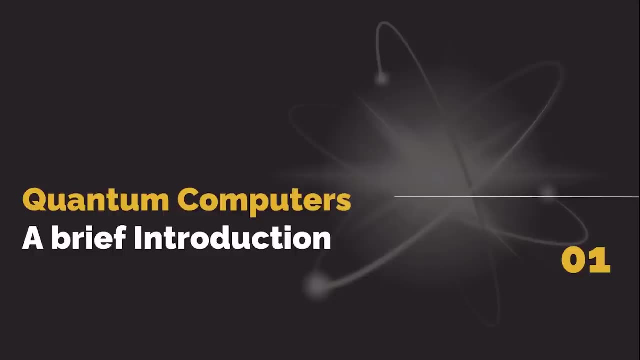 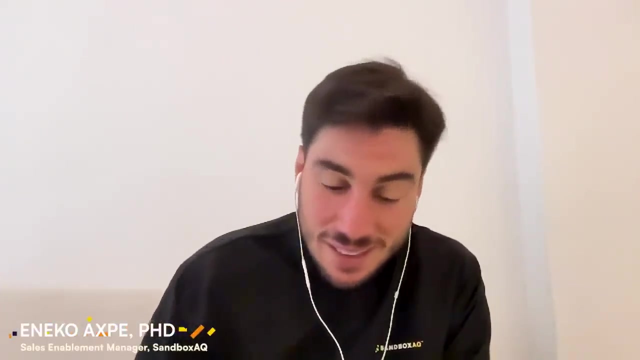 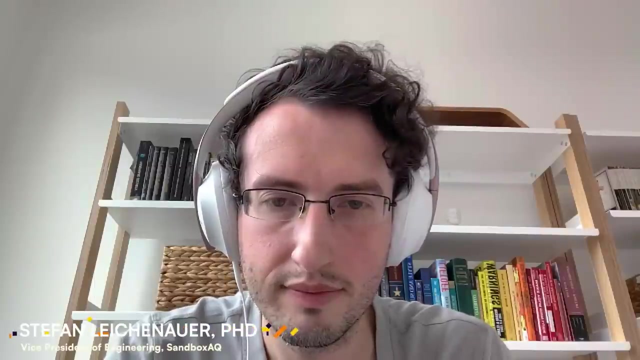 We are going to learn about quantum computers today. My name is Eneko Aspe, I'm the Sales Enablement Manager at SandboxAQ and today we have Stefan Leikenauer with us. He is a physicist and the VP of Engineering at SandboxAQ. Hello Stefan, Hello Eneko. 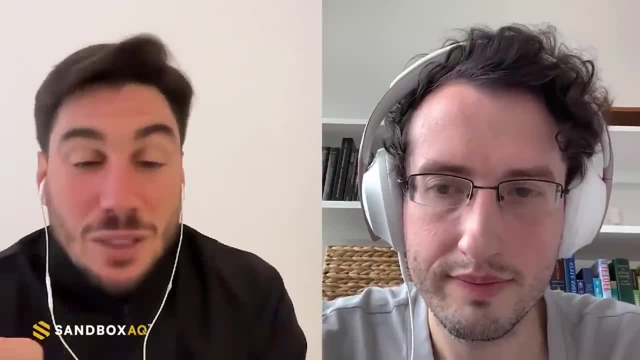 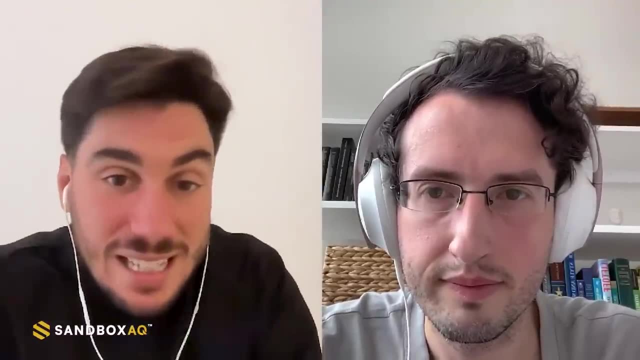 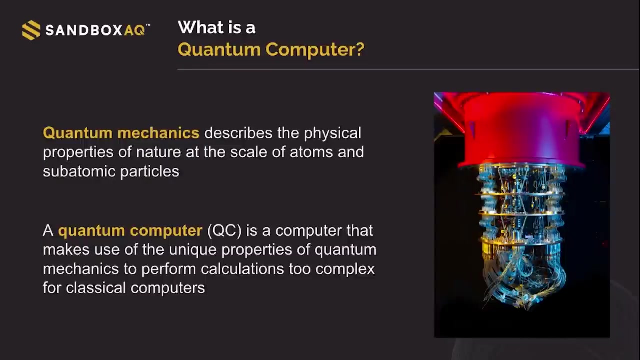 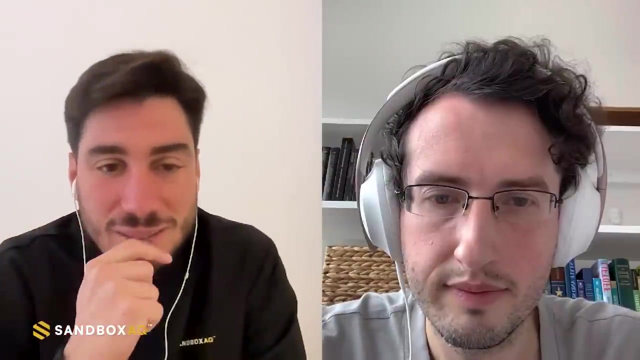 We're going to start talking about quantum computers. We're going to introduce them briefly. First of all, we need to say that quantum mechanics describes how the physical properties of nature behave at the scale of atoms and subatomic particles. What is exactly a subatomic particle? Well, a subatomic particle, I mean, we learn in school, right? 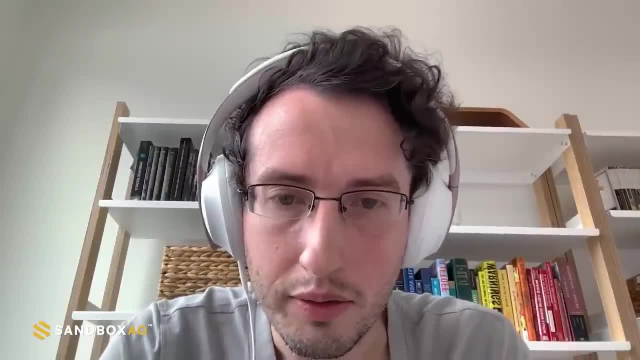 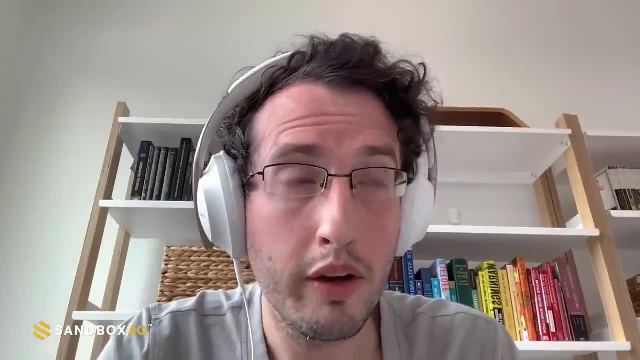 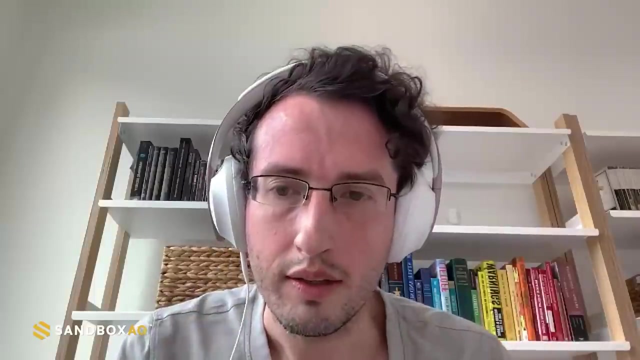 that atoms are made of, you know, protons and neutrons in the nucleus and electrons around the nucleus and things like that. And it was discovered even more than a hundred years ago now that our ordinary ways that we talk about motion and dynamical laws just don't work for. 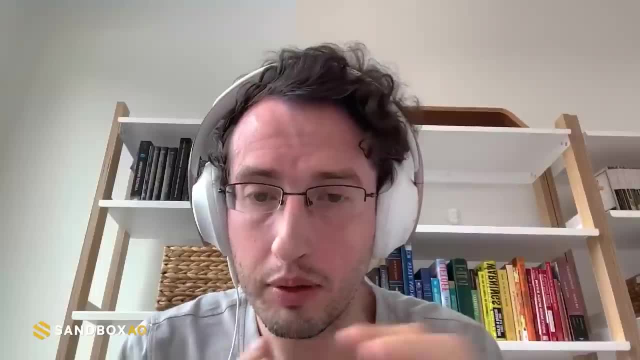 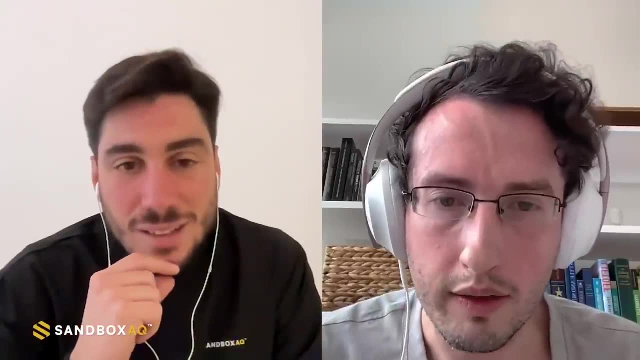 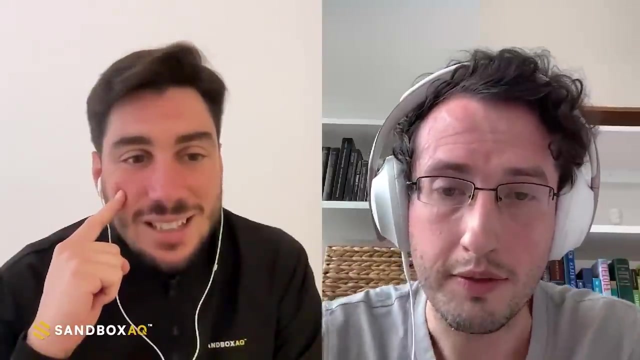 those kinds of particles, Either the atoms themselves, the electrons, the protons, the neutrons, or even smaller things like quarks that you may have heard of, And so that's when people use quantum mechanics to really figure out how those atoms worked, And it's been a huge success. 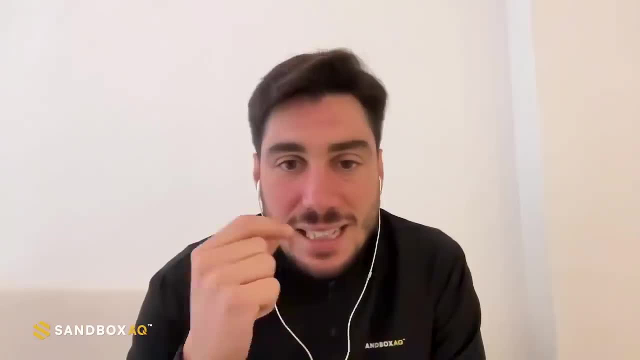 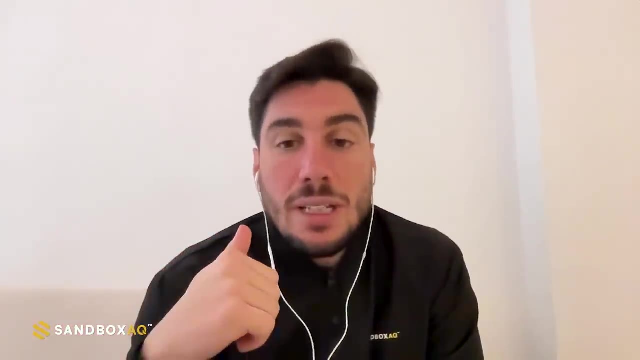 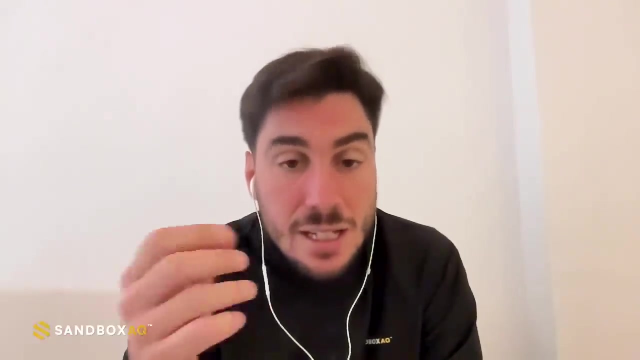 for the last hundred years. So what we are saying is that these particles, at this tiny, tiny scale, they behave in a unique way, right, And what quantum computers do is to make use of these unique properties of quantum mechanics to perform calculations too complex for classical computers. 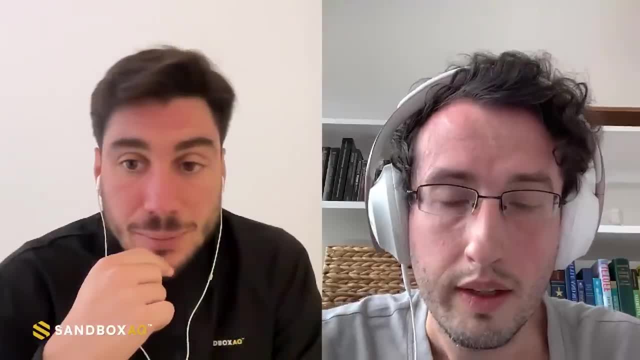 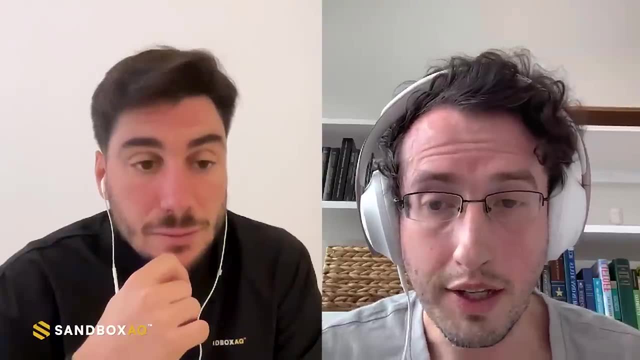 Can you tell us a little bit more about this? Yeah, yeah, that's exactly right. So the rules of the game when you're talking about subatomic particles are a little bit different, And actually the truth is that even you know you and me obey those same kind of weird quantum laws. 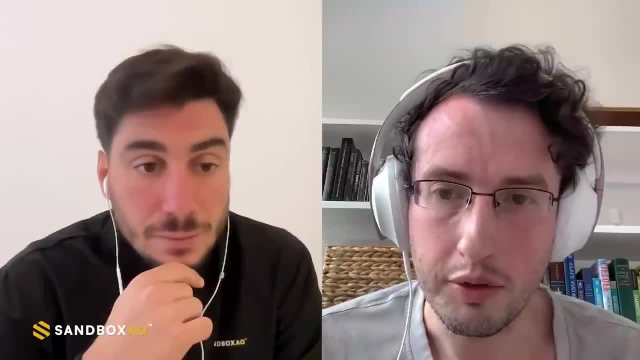 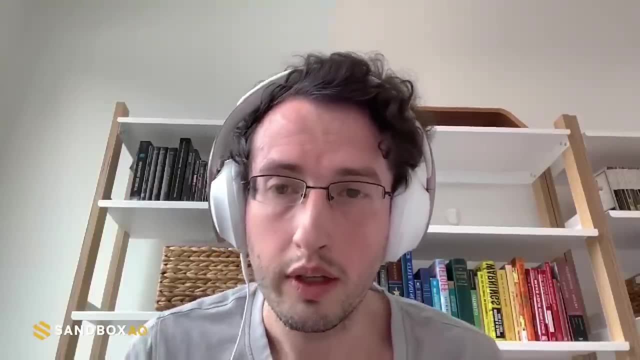 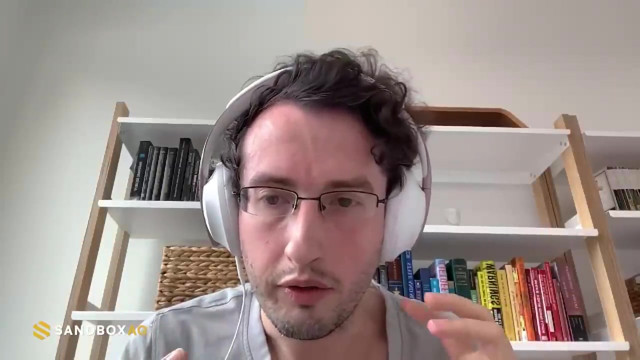 It's just that when you have, when you're very large, you sort of don't notice that things are a little bit strange. But at the very small scale, usually when things are also very cold although necessary, you notice that the rules are a little bit different. You have sort of quantum mechanical. 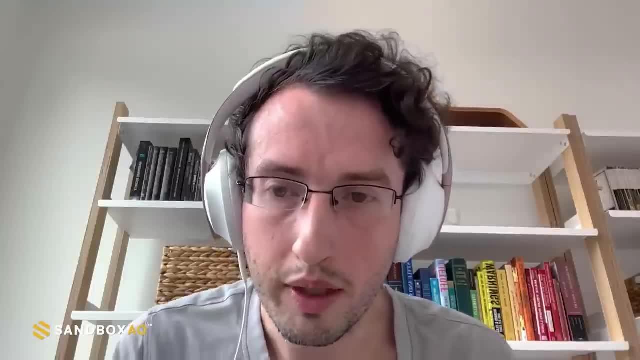 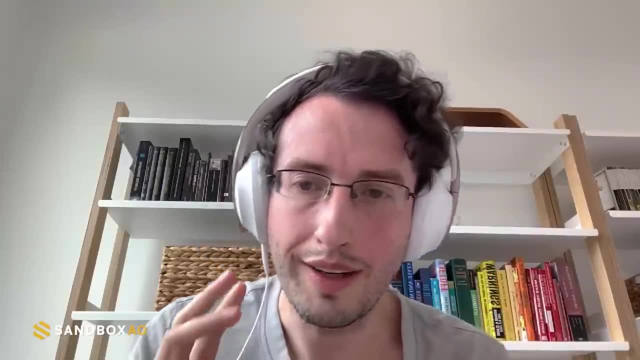 things that can happen, the details of which are probably beyond the scope of our conversation here, But it means that the you know different things like superposition and entanglement. you know people like to use words like: the particle can be in, you know, can be in one state. 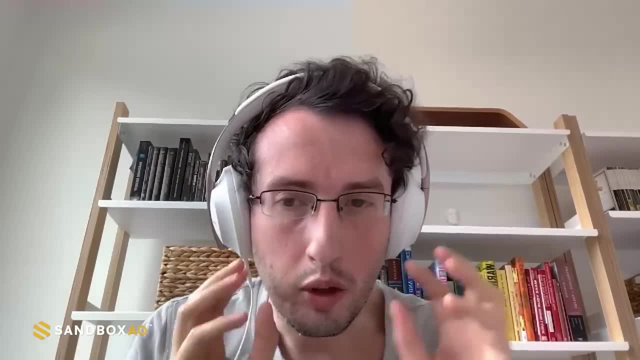 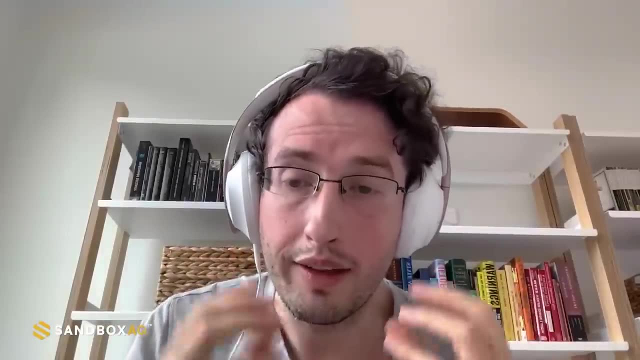 or another state, or maybe two states at the same time. That's a little bit sloppy language, but it's the usual. that can't happen classically, can't happen in the ordinary world, at least as we usually think about it. And if you can take advantage of those weird properties, then it. 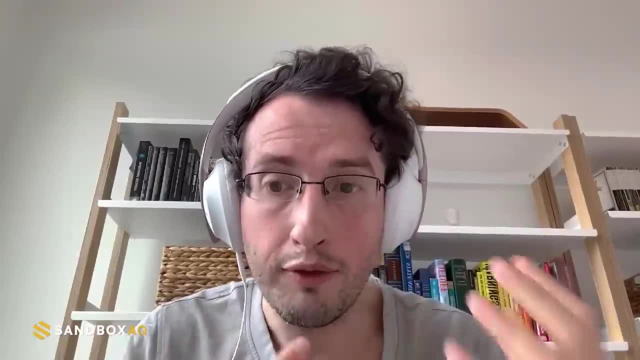 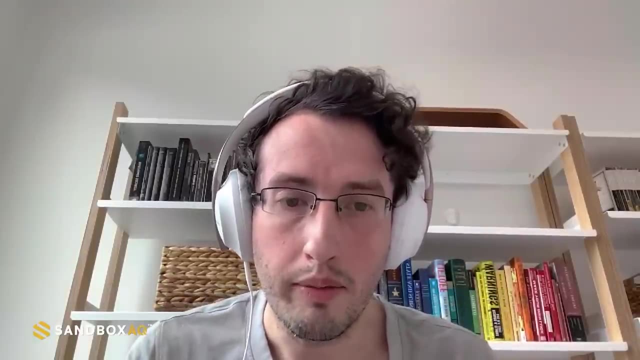 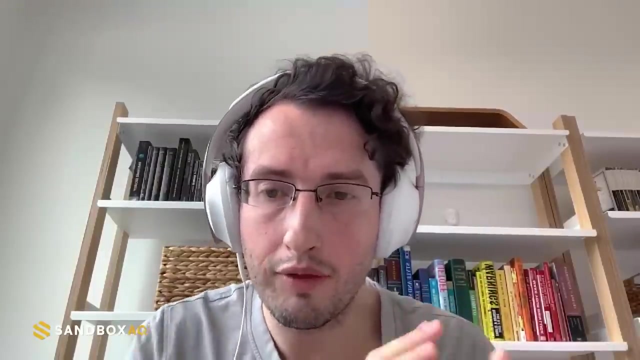 allows you to do things to do like information processing, using these kinds of special rules and these special ways that systems can behave that are not part of the ordinary rules And, if you can take advantage of those, it allows you to do different things like a different set of. 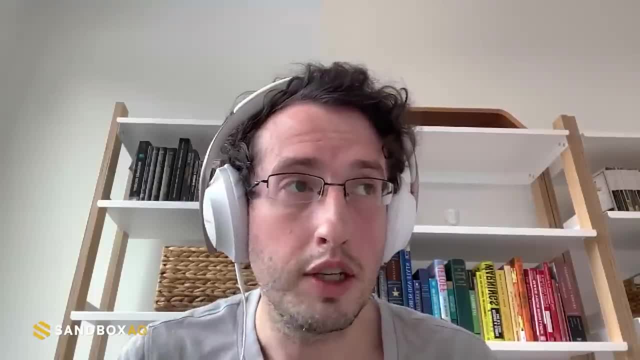 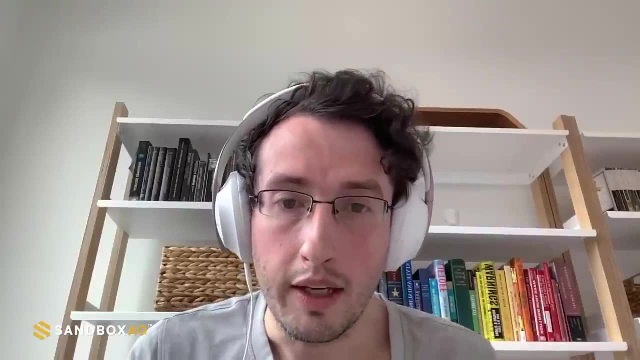 operations than you used to be able to do. I like to use an analogy with calculators. right, If you have a basic calculator, you can add, subtract, multiply, divide, things like that. And if you get a more advanced calculator? 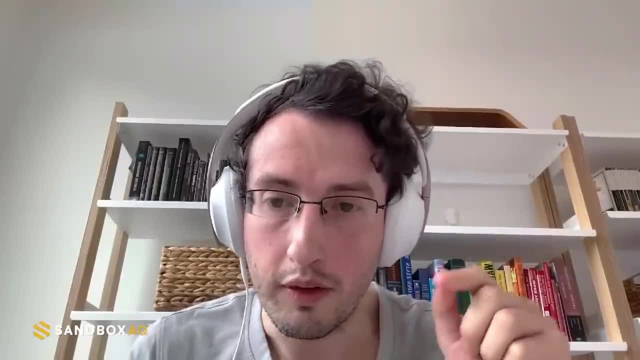 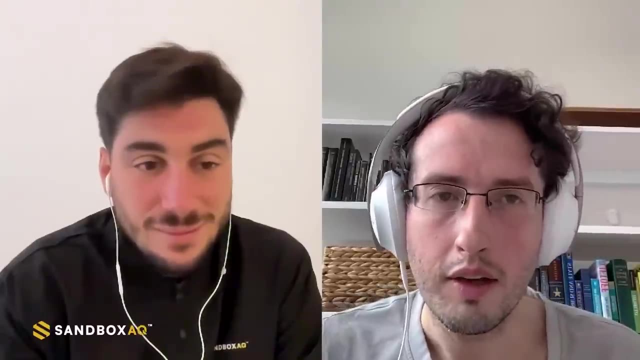 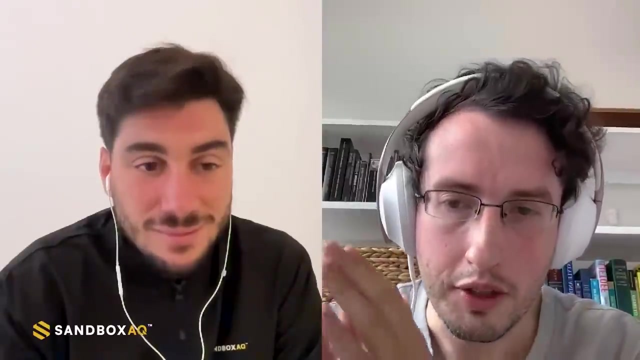 like a scientific calculator. then you can automatically take square roots and do exponentiation and even fancier calculators that you do calculus like integration and differentiation, fun things like that, And all of those operations. it's like you increase the list of operations you can do, but they're all built out of addition, subtraction, multiplication in. 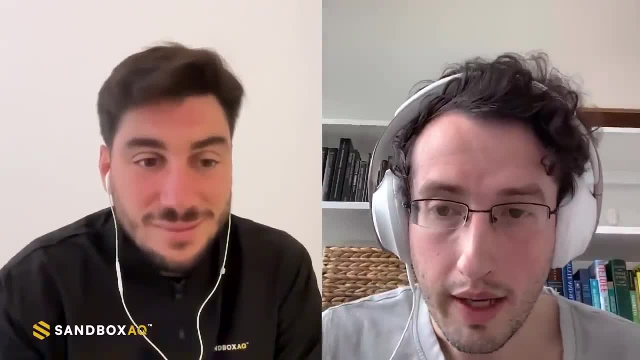 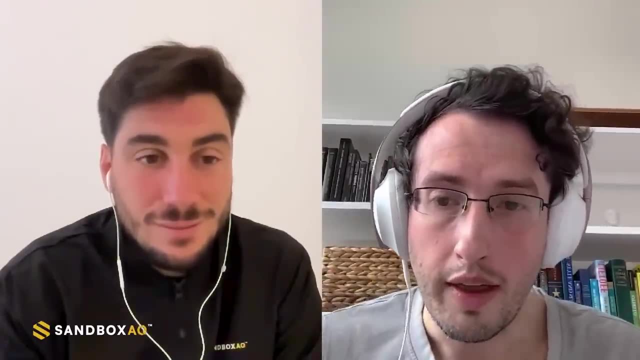 some way right, But they're just getting more and more complex. Quantum mechanics is like, and having a quantum computer would be like having a different sort of calculator with a different set of buttons that are not built out of addition, subtraction, multiplication and division. It's just. 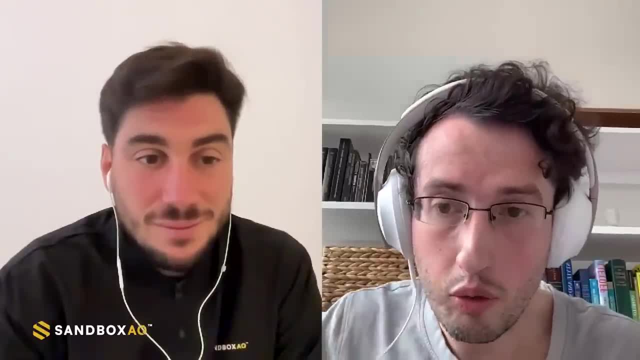 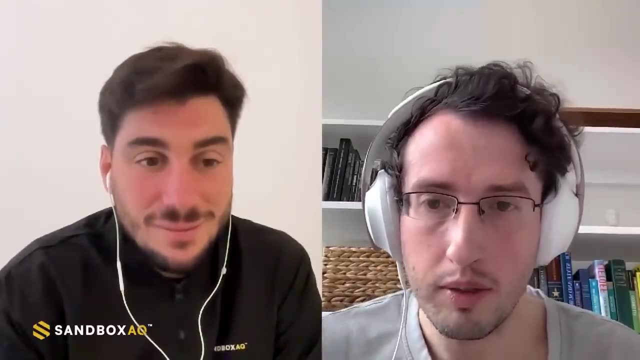 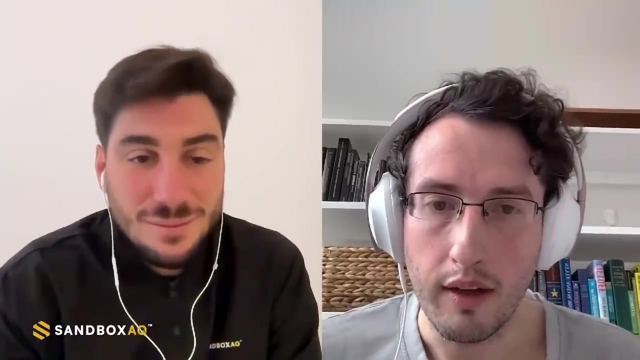 they're very complicated things that are just new. They're new by themselves. You could try to model them using addition, subtraction, multiplication, division, but it would be very inefficient And the quantum computer sort of performs those new kinds of operations natively. And learning how to use those that new set of buttons is really the 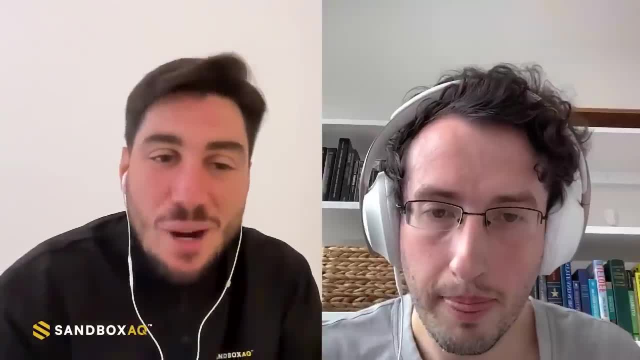 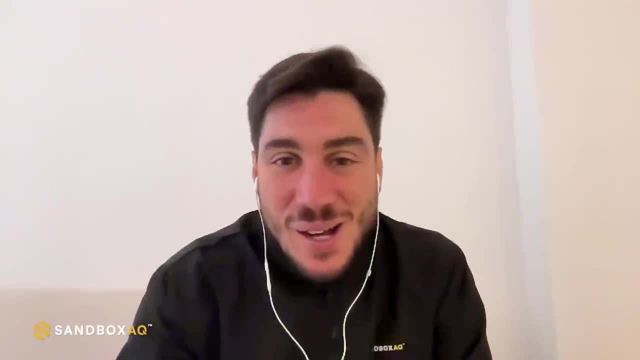 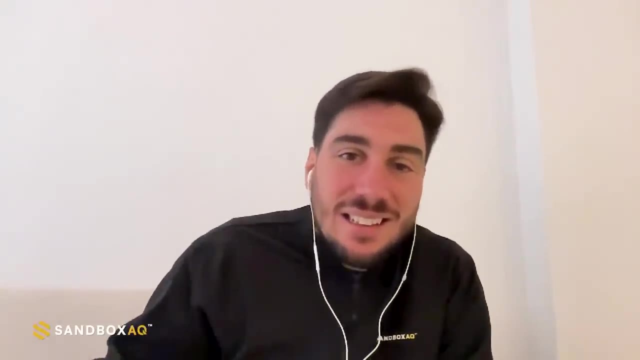 challenge, but it's also the opportunity. Awesome. So we have a brand new computer with brand new physics that are explained through the quantum mechanics. Perfect, Let's talk about a little bit the differences between classical and a quantum computer. So we all know that. 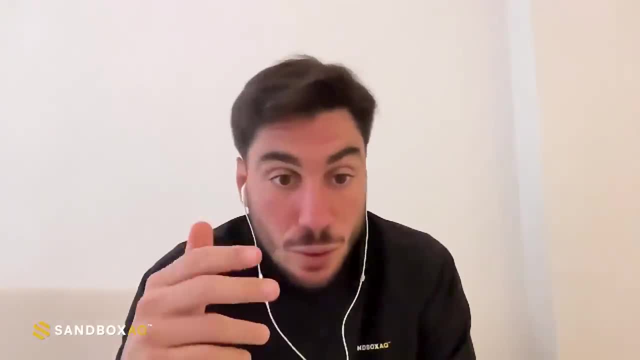 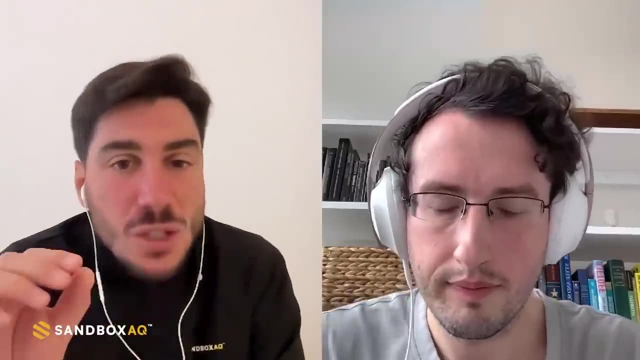 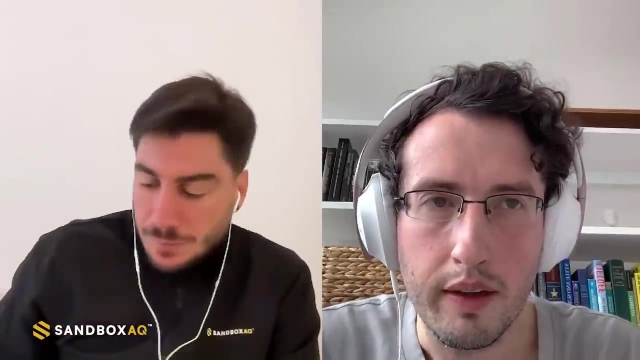 classical computers calculated with bits, so zero and ones. but apparently we have some kind of quantum bits or qubits, And that's what we use in quantum computers. Can you tell us a little bit more about that? Yeah, Yeah, So you'll often find that in the quantum context people take a normal word. 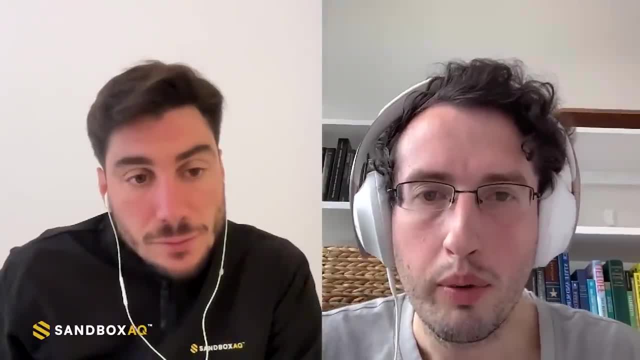 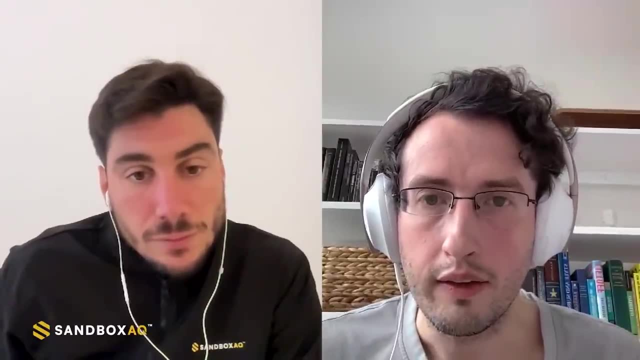 and then add a Q to it or something to emphasize that it's quantum. But really the only difference between a qubit and a bit from one point of view is that a qubit it says: take a bit and then try to apply quantum rules to. 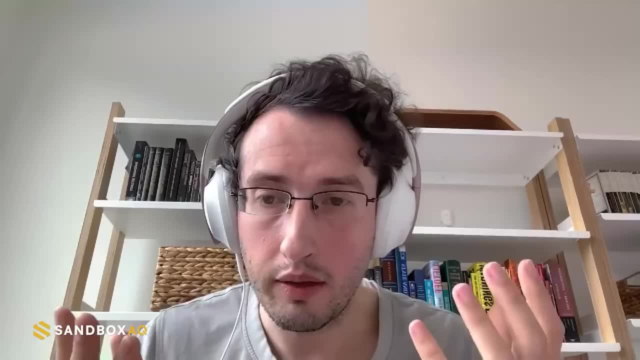 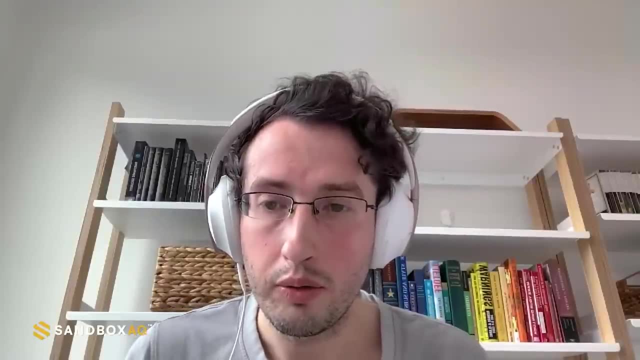 it So a qubit like a bit. it can represent a zero or a one, just like a bit. But if we're using the rules of quantum mechanics then you can also do these things called superpositions. So you can say the qubit is in zero plus one, And that's a little bit weird. What does that? 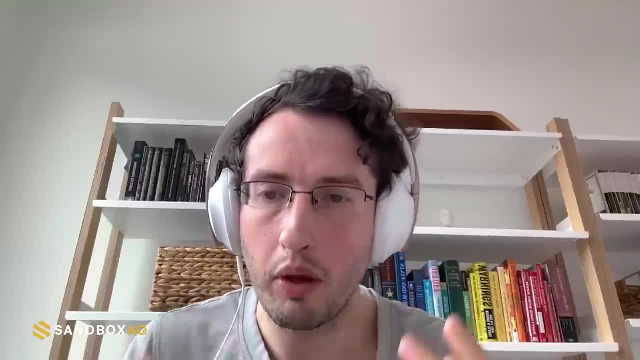 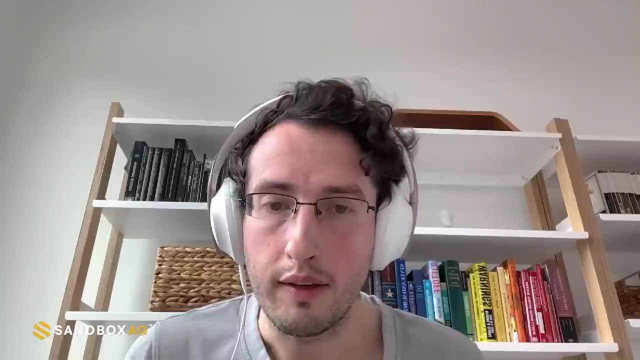 even mean Zero plus one or zero minus one, And people often say things like it can be zero or one at the same time. That's the language people try to use, But really what it means is that the qubit is neither zero nor one If you looked at it and tried to see, okay. 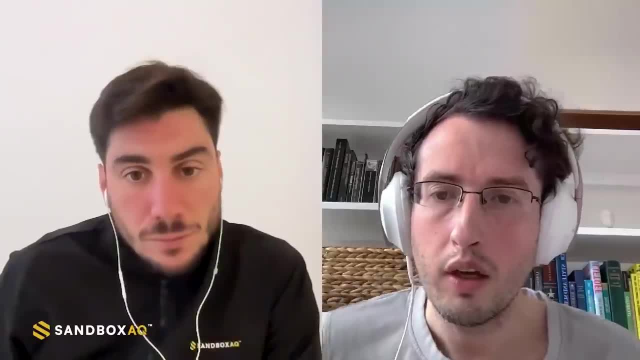 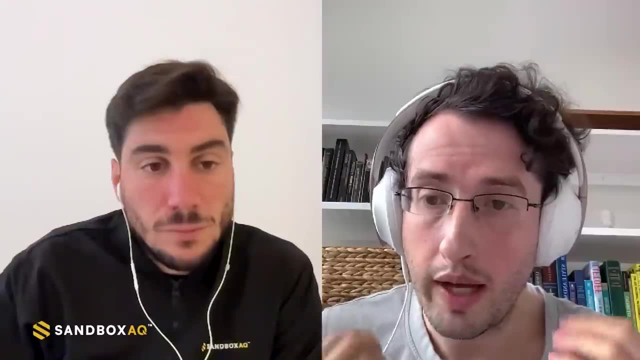 what is it? Is it a zero or a one? Let me just look at it and see. Well, you would see either zero or one, but which one you see is random. It's determined only at the time when you do the measurement, And so 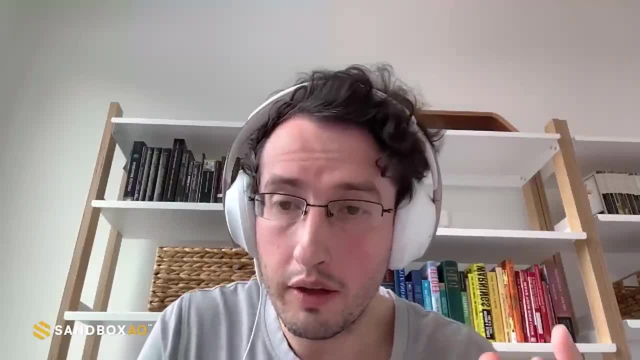 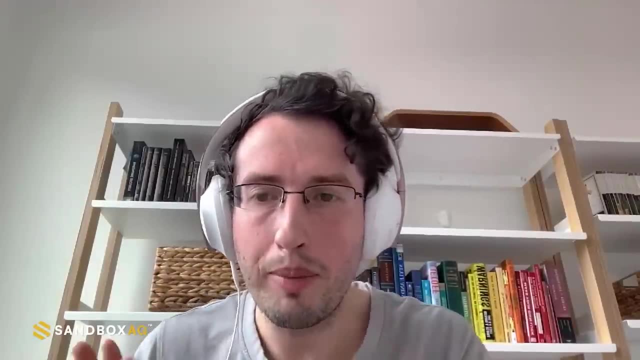 there's a little bit of probability associated with it, And what is the likelihood of getting zero? What is the likelihood of getting one? That's determined by the particular nature of the superposition, And so there are many, many possibilities for what the state of the qubit 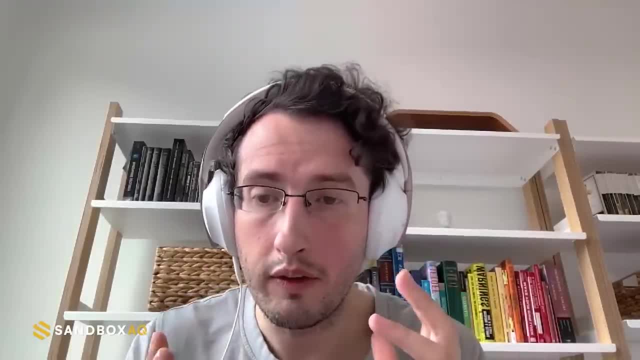 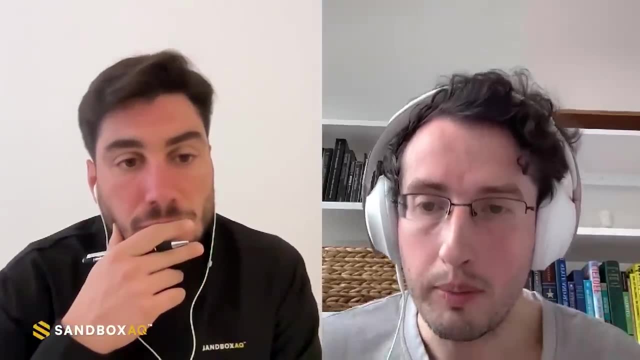 can be besides just zero or one. It can be in one of these mixture kind of states, superposition kind of states, And that's where a lot of the power of quantum mechanics comes from is taking advantage of these new kinds of states. 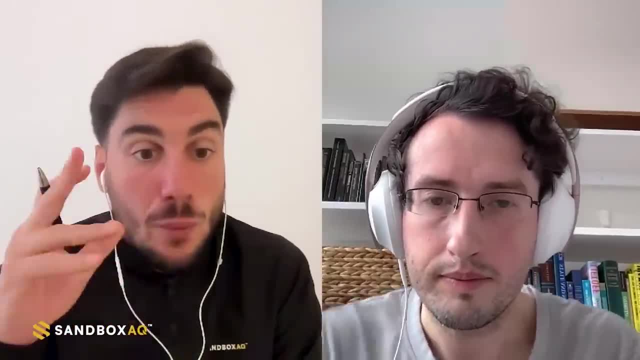 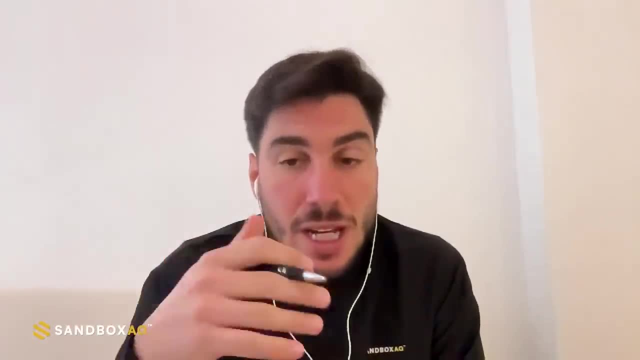 And that's what give us like a new power. let's say right, Because we know that in classical computers power increases linearly with the number of transistors. However, in quantum computers, power increases exponentially with the number of qubits. right? 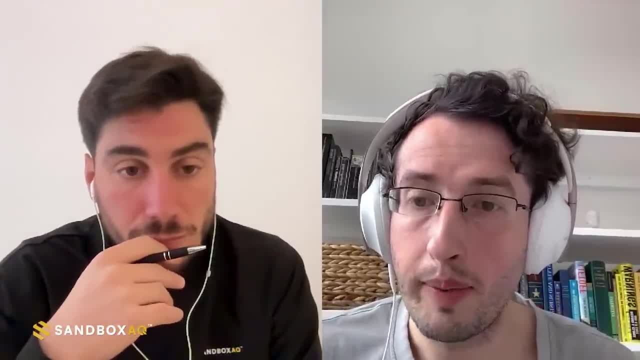 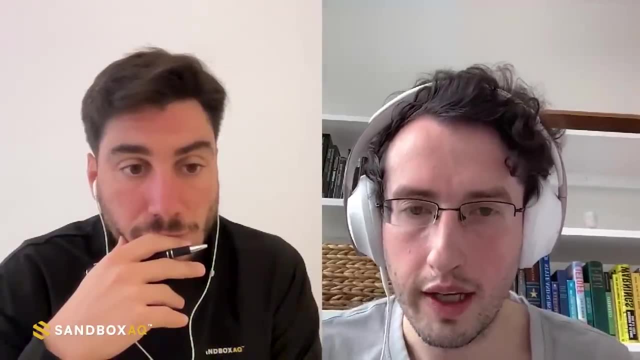 Yeah, So I mean what that means is it comes back to this idea of let's try to. what would we do if we didn't have a quantum computer, If we just had a classical computer? but we wanted to try and take advantage. 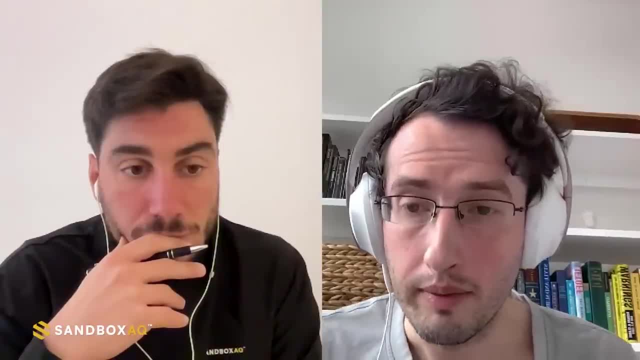 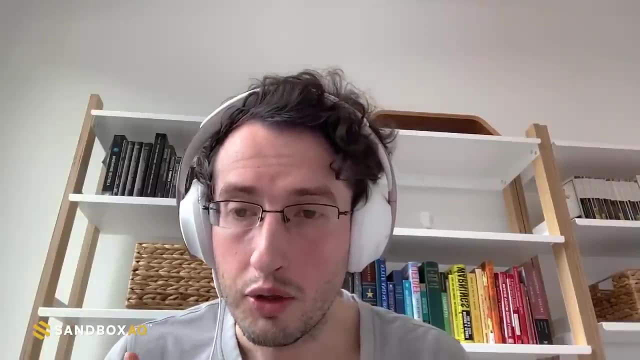 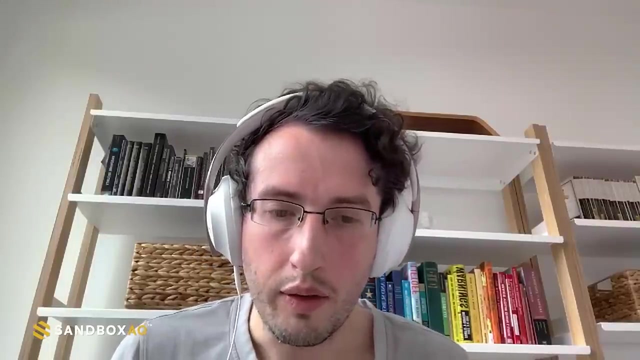 of these quantum algorithms anyway. Well, you can always just try to solve the quantum equations on a quantum computer and try to pretend that you had a quantum computer. It's just like solving the equations that people wrote down 100 years ago, And the problem is that every time you add 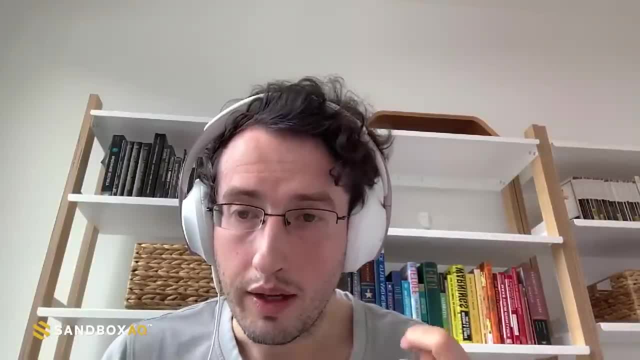 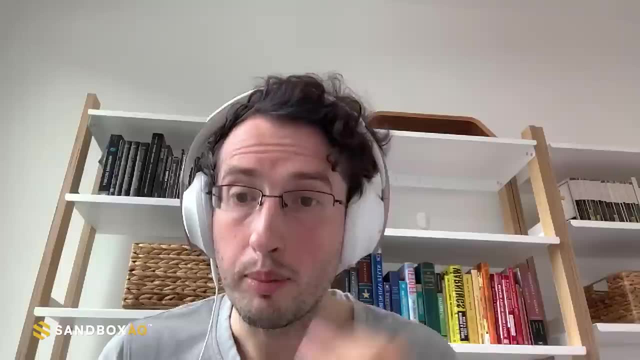 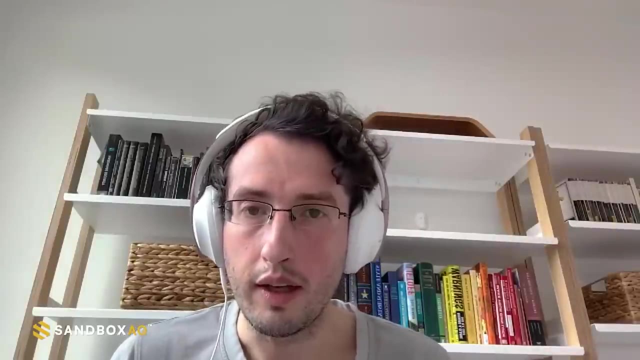 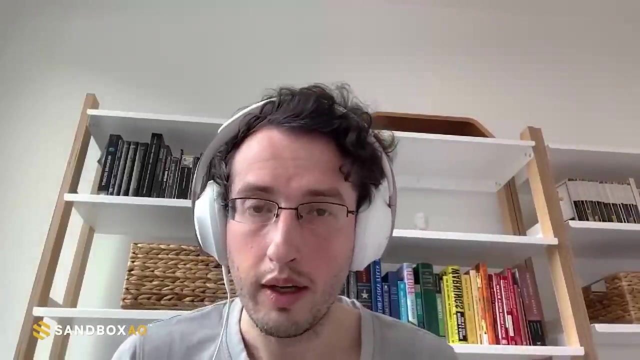 a qubit to the quantum computer, the classical power that would be required to simulate what was happening in that quantum computer would double, And so that's how this exponential growing power comes about. It's sort of, if you think about how much classical emulation would be required. 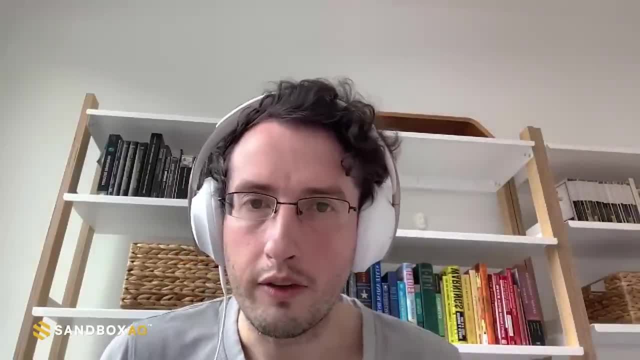 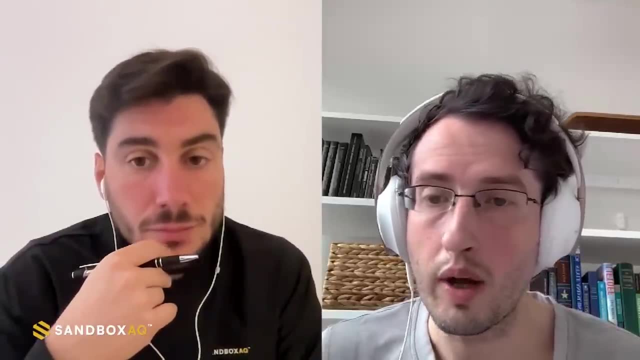 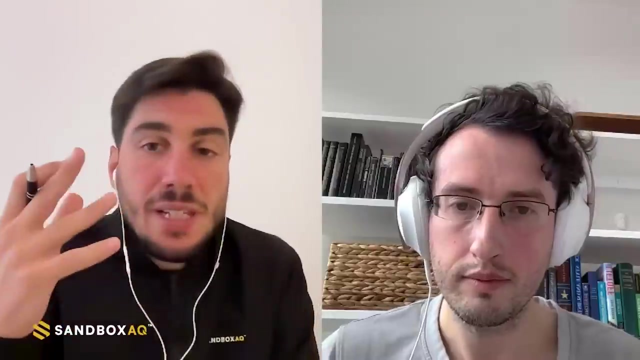 it just grows, It's just out of control. And so very quickly, very quickly, you end up in a situation where it's impossible to even try to duplicate the quantum power using a classical computer. so, basically, we have a very, very powerful computer. in the case of 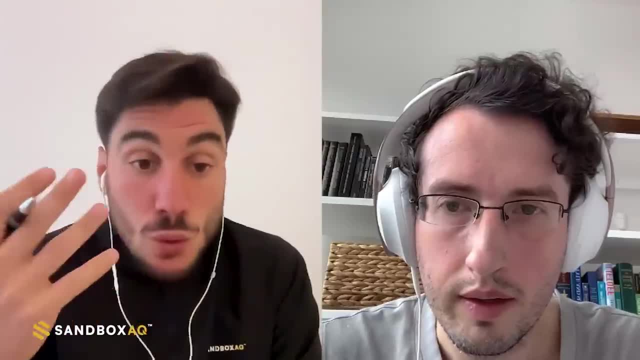 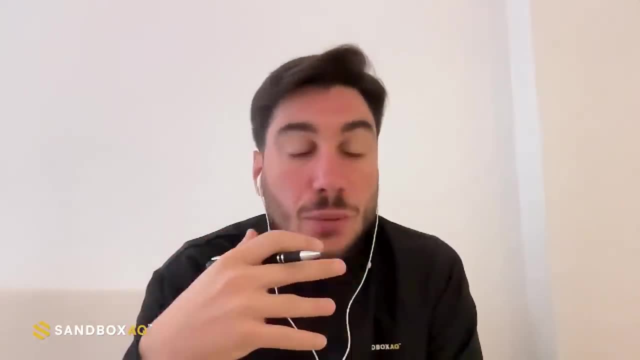 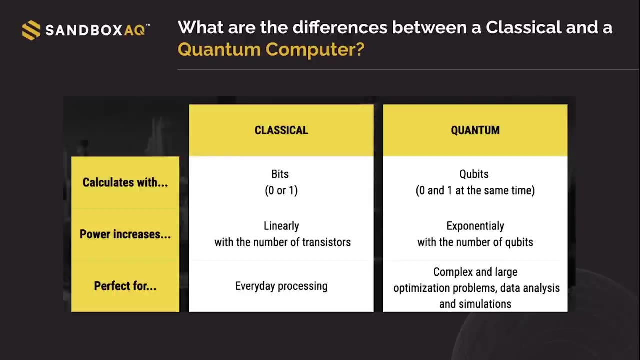 the quantum computer. however, the use we're gonna give to quantum computers is not in the everyday processing. that will be more set for classical computers, right? so we say we will use quantum computers in certain cases, right, when we want to solve optimization, optimization problems that are complex and very large machine learning simulations, but only in these cases, right. 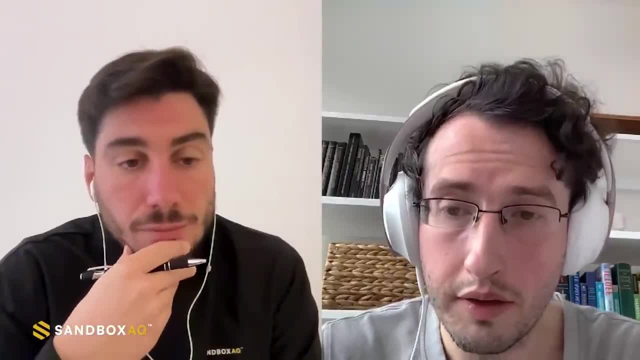 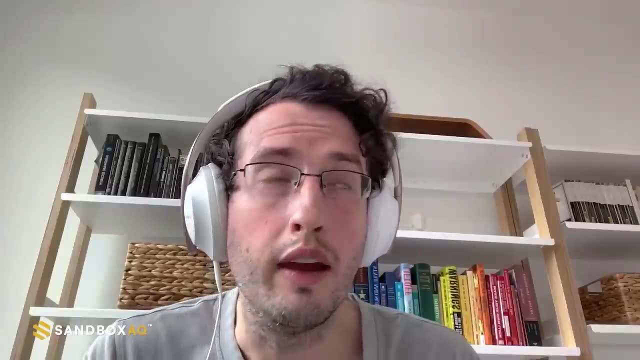 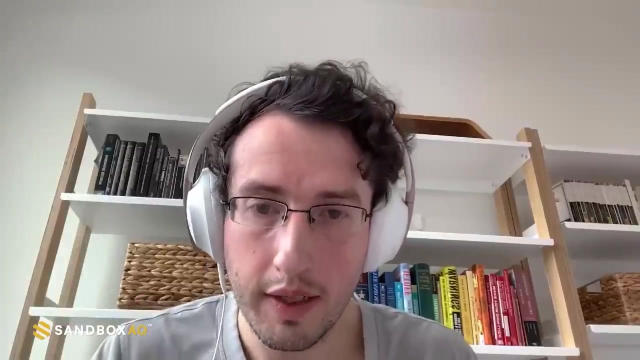 yeah, yeah. so quantum computers. if we come back to my analogy from before, we have these new buttons on our calculator, right that let us do quantum things. and you should ask yourself: okay, what are these new quantum operations good for? like can i use them to solve every problem instantaneously? 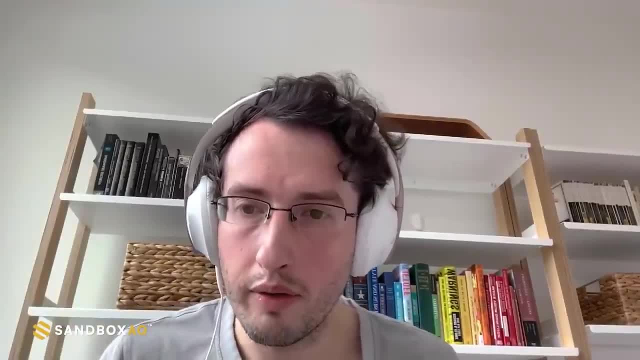 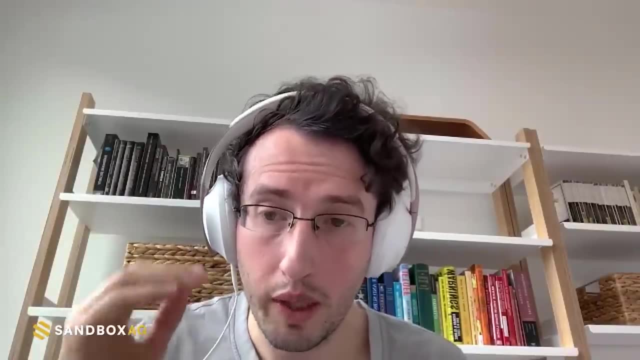 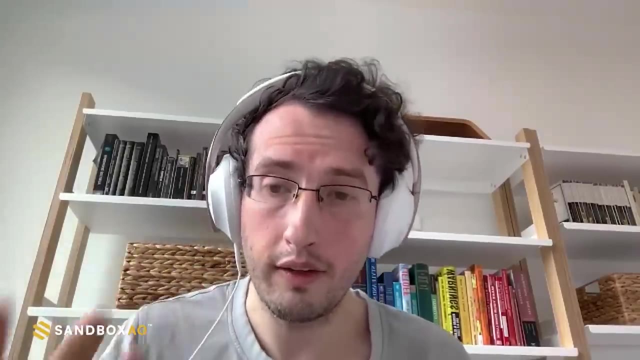 the answer is no. um, actually, the number of you know. if we make a list of all the things that we know for sure that quantum computers um are good at and that we can leverage the quantum power for, uh, it's actually not a very long list. there are a few things that we suspect are good ideas. um, you know one thing, uh, that like 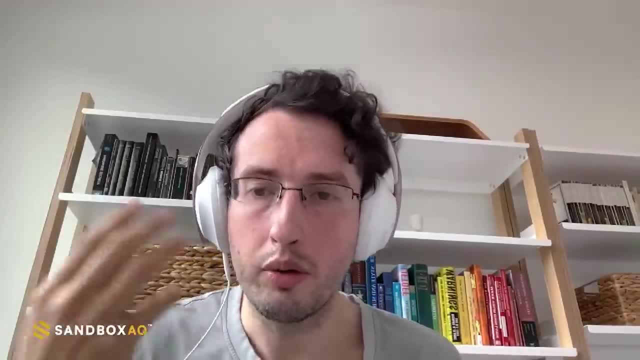 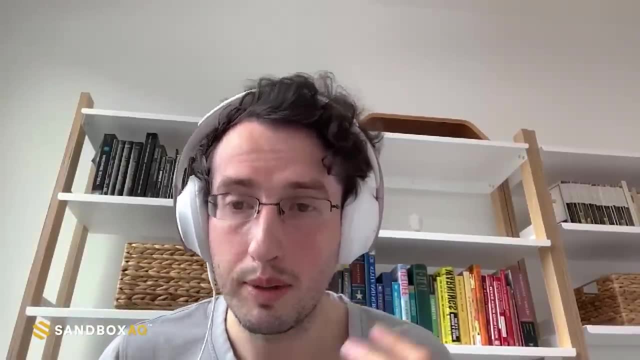 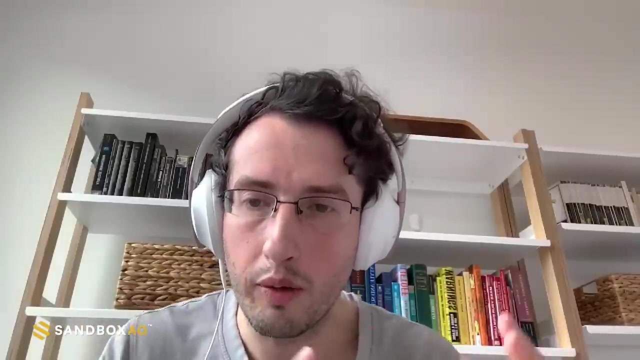 chemistry, for example, things that are inherently quantum. also, people strongly suspect that in the not too distant future we'll be able to get some kind of advantage looking at different kinds of optimization problems and things like that, and certainly we can talk about what. what are the particular algorithms? 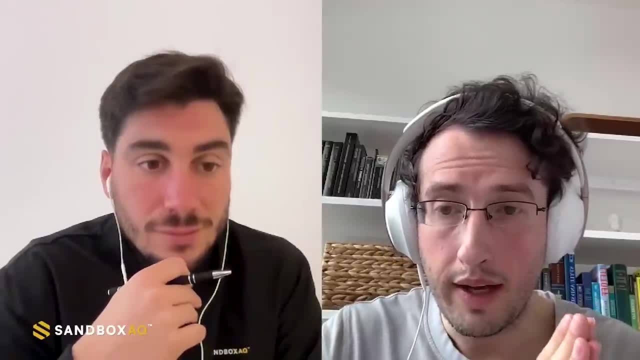 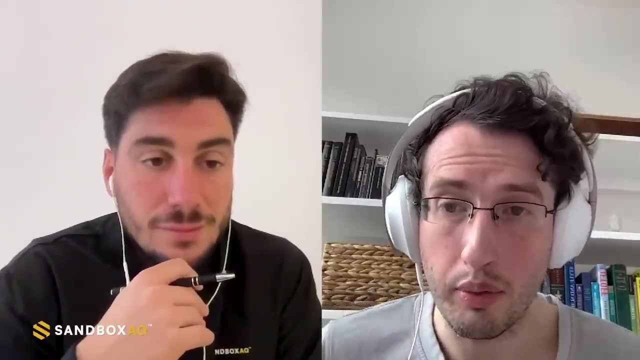 that we know. but if a quantum computer is not, if you can't take advantage of those special quantum properties, if the if the quantum computer is not especially good at your problem, then you should not be using a quantum computer got you. it would be like it would be like killing a mosquito with. 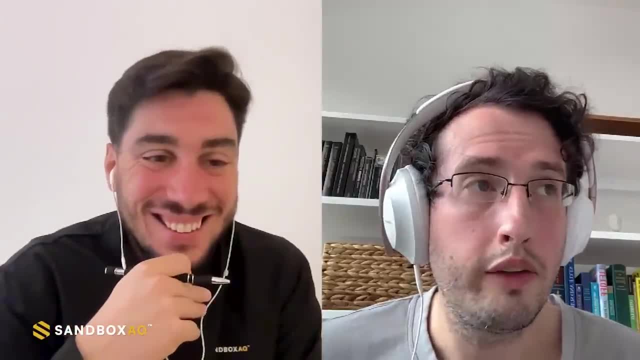 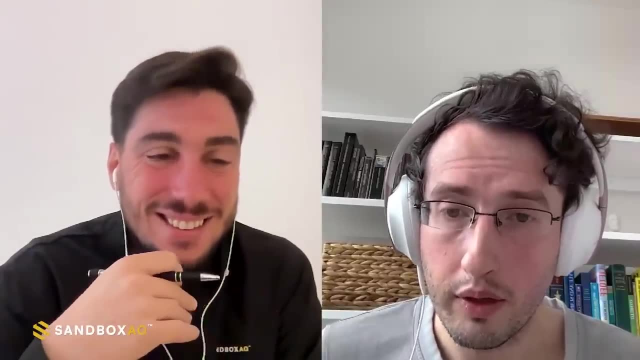 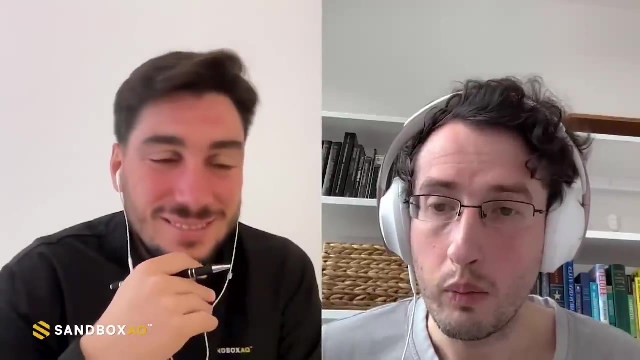 a bazooka or something like this. right it, i would say it's, it's kind of, it's even worse than that. if you, if you, if you tried to use a quantum computer for ordinary stuff, like to say stream a movie or something, um it would, it would be just extremely slow, right a quantum computer. 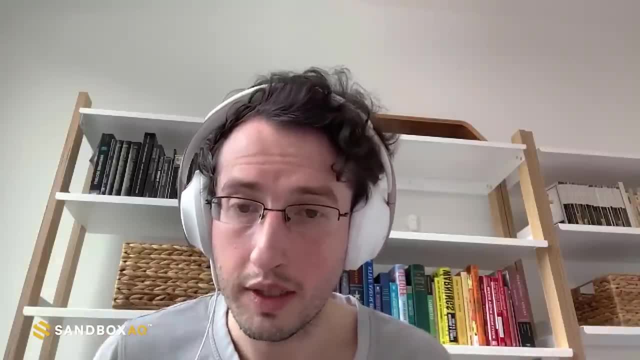 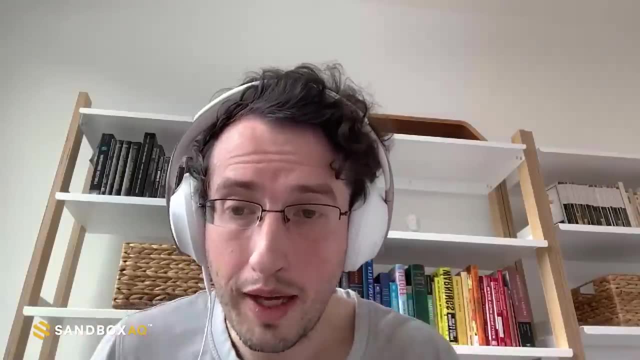 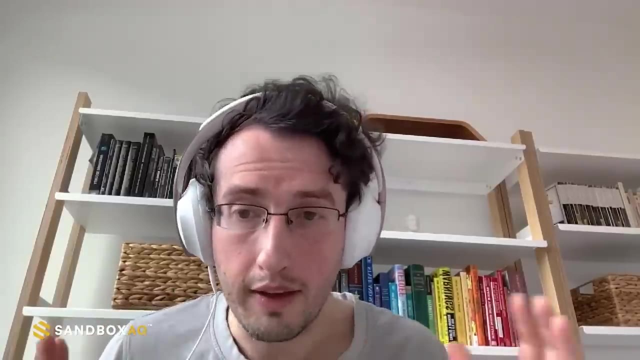 is a quantum computer, operates at a much slower clock speed, for example, than a classical computer. it does many fewer operations per second. so if you're not taking advantage of its special properties, you just shouldn't use it, because it would. it would be slow and expensive. the it gets it despite the fact that it's slow in operations per second it can. 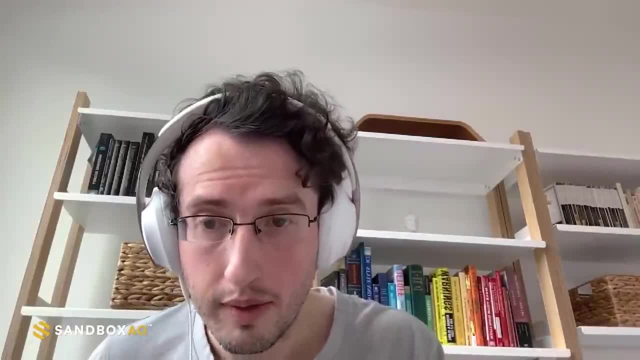 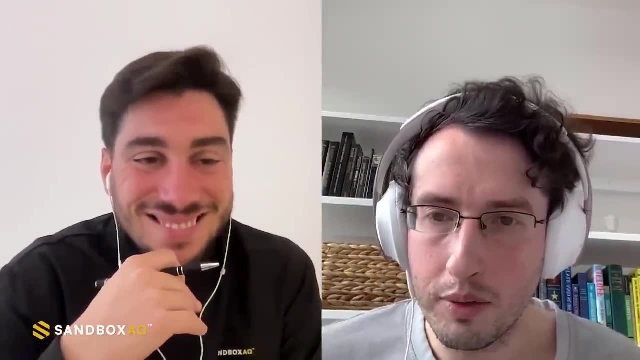 solve certain problems with many, many fewer operations, and that's where it gets its advantage. that's why it would be useful looking at it so it so yeah, it'd be like killing a mosquito with a bazooka in slow motion. understood so everyday processing classical computers. 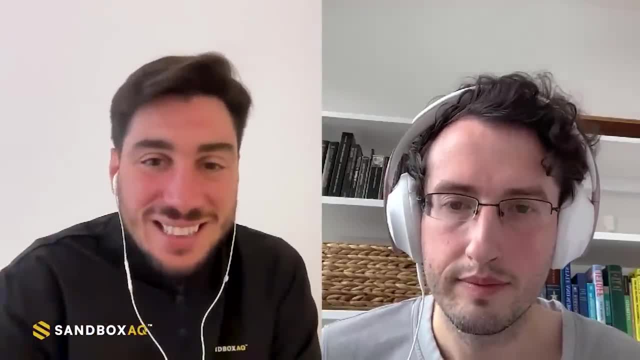 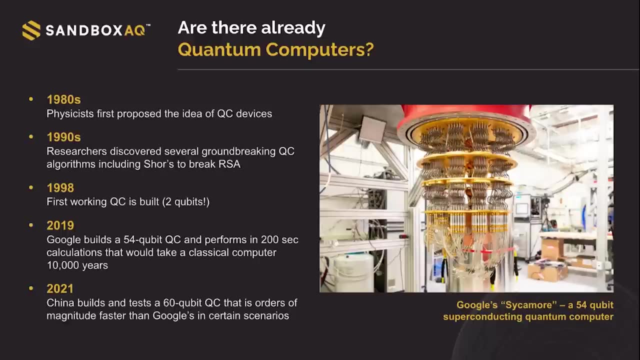 very complex and large problems quantum computers understood. this is a timeline of the quantum computers, even if it is surprising. already in the 80s physicists proposed for the first time the idea of quantum computer devices. but there was a ground breaking point when short published the paper in 1994 where he described an algorithm that 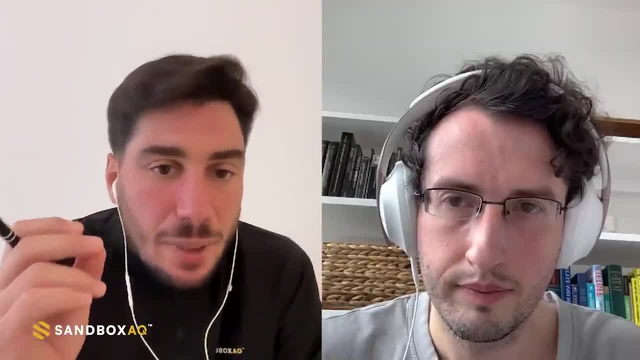 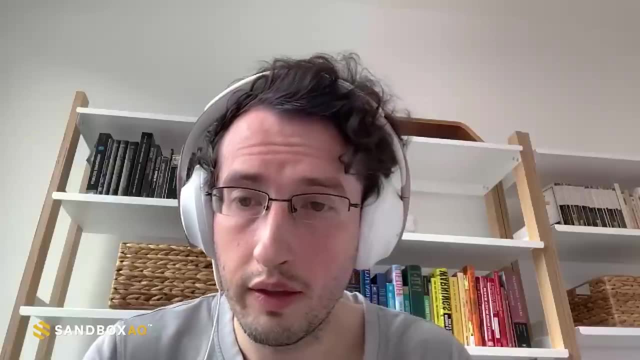 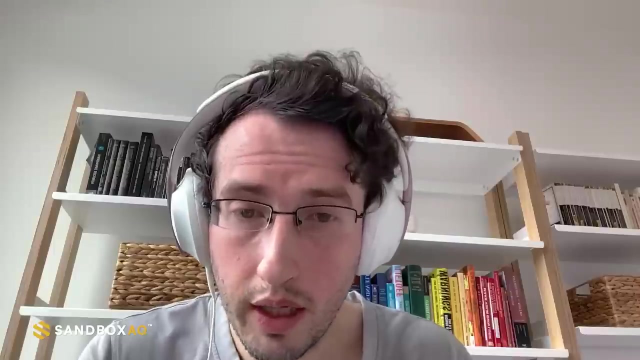 is able to break rsa that paper so important, stefan, yeah, so back in the early days before, sure. so in the in the through the 80s and into the early 90s, um, the main use case for quantum computers that people were thinking about was using a quantum computer to simulate quantum physics. right to understand what was. 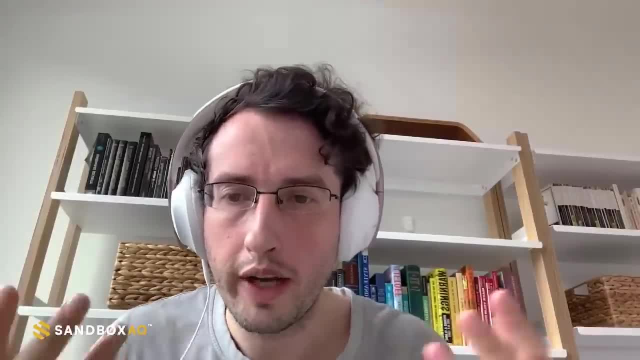 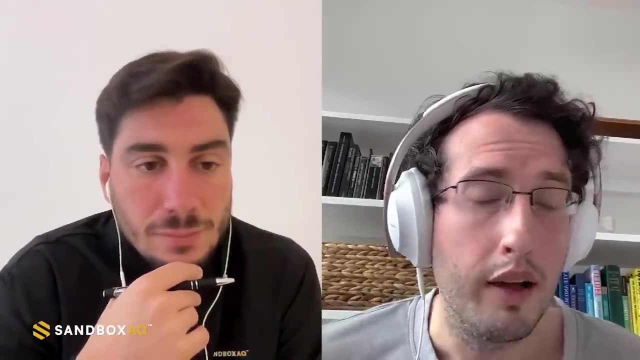 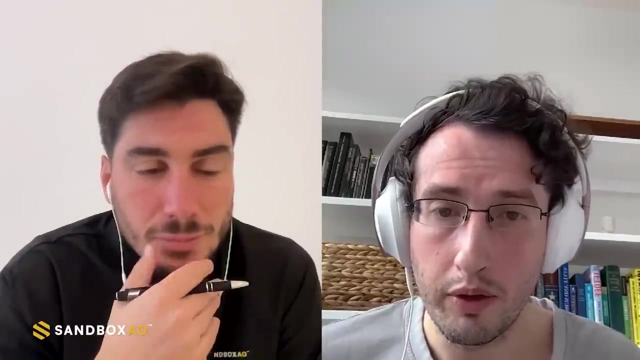 happening for subatomic particles, for example, because those are inherently quantum and so you know, maybe use a programmable quantum computer to simulate what's happening and learn something. that's interesting. david deutsch showed in 1985, at least in principle it was possible to think of these quantum computers. 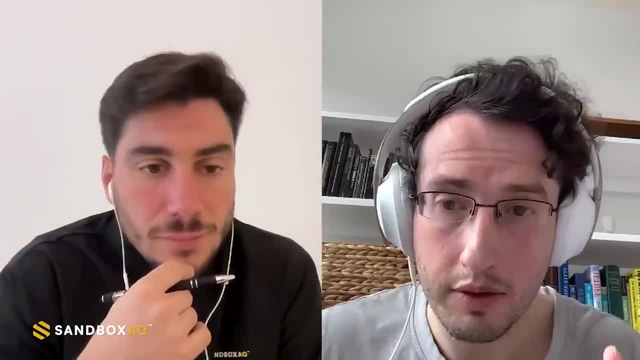 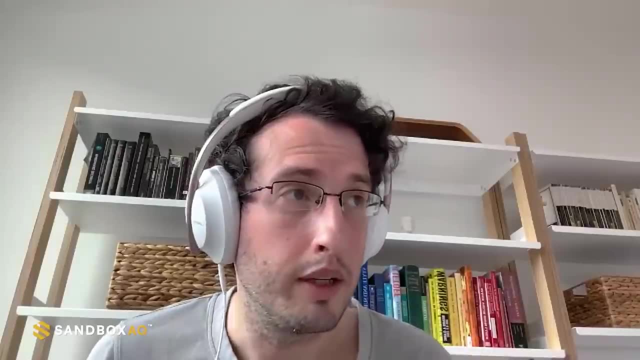 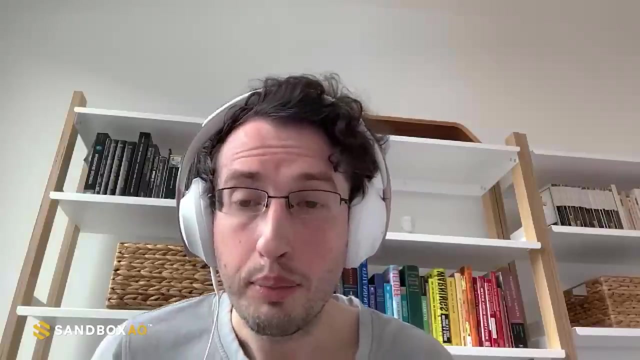 as not just simulators of physics but as computers that could be programmed and do things, and he demonstrated, at least in principle, with some follow-up work with collaborators also, that there would be problems like logical type problems that could be solved in principle faster on a quantum computer than on a classical computer, but nothing. 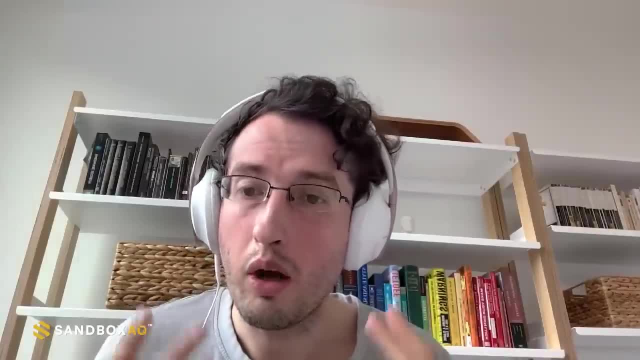 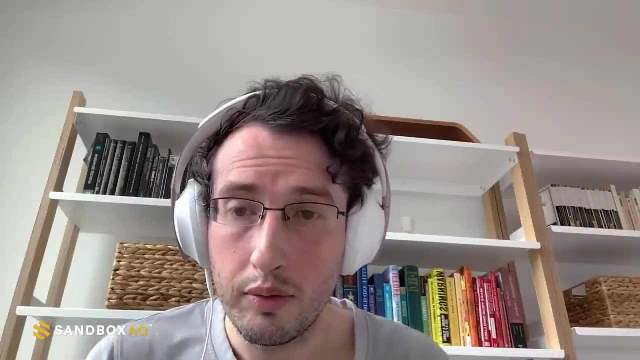 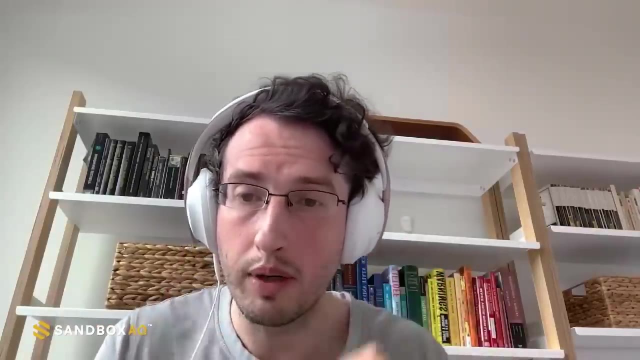 that was really nothing that really caught people's eyes is like: oh yes, this would be really useful. the difference in 1994 is that peter shore showed us how to uh factor numbers, large numbers, how to take a large number that was, say, a product of two large prime numbers, and i just give you the. 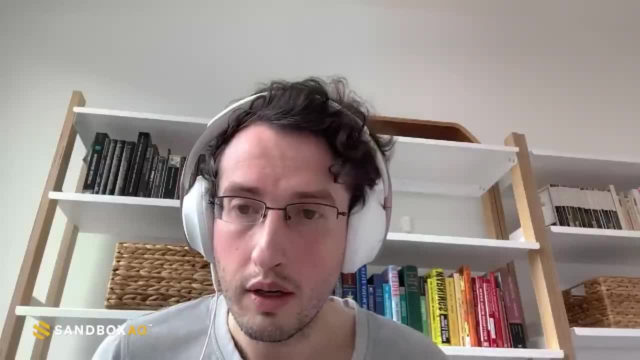 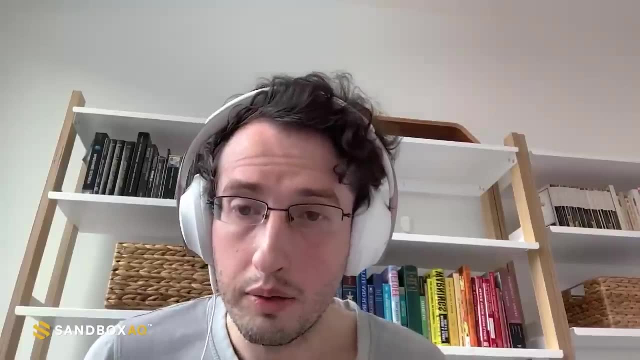 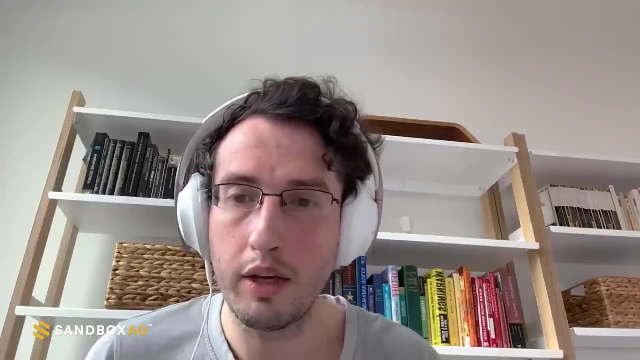 the that, that product, and i ask you, what are the numbers that are its factors? find me the two prime numbers that i multiplied together. and that's a problem. and he showed how the quantum computer could solve that problem very quickly. um, much, much, much, much more quickly than anybody. 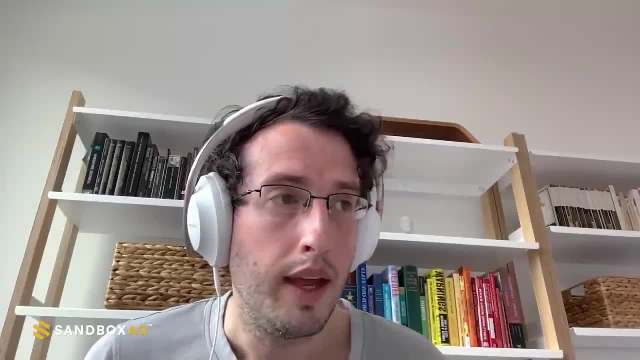 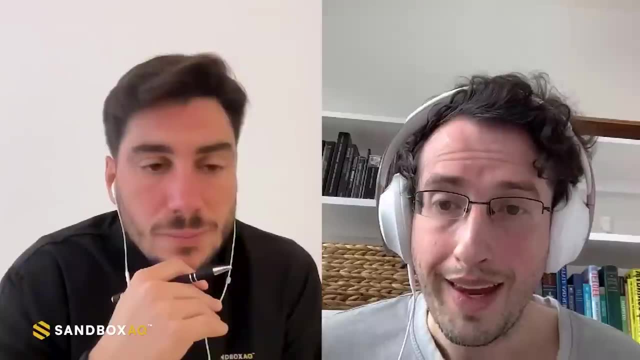 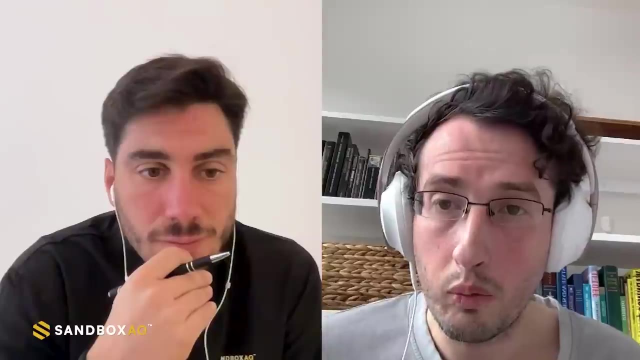 knows how to do, even to this day, using a classical computer. and that problem is special because that's a problem people have been trying to solve for a very long time, and the fact that that problem is hard to solve on ordinary computers is the is the reason why um rsa, rsa crypto system is. 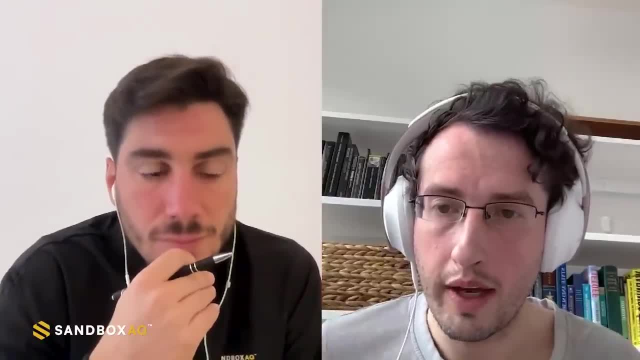 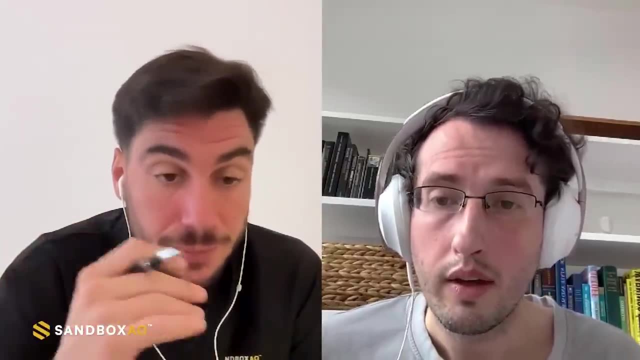 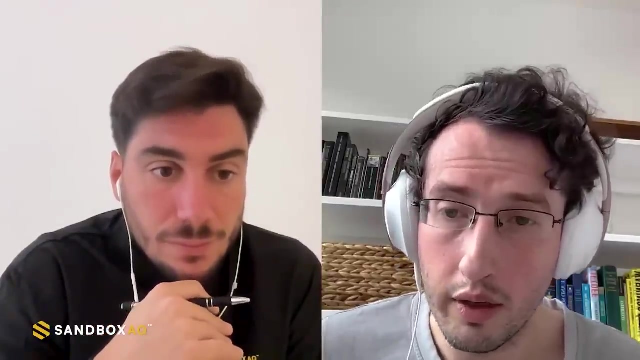 considered secure? uh, because it's. you know, the security of that cryptography is based on the fact that that problem is hard, which is which is the cryptography that we use every day. that's right. that's right. so we use rsa, which is based on the factoring of hard of large numbers. we also use uh- elliptic. 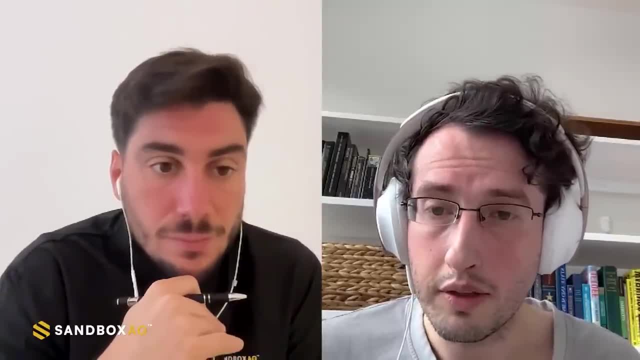 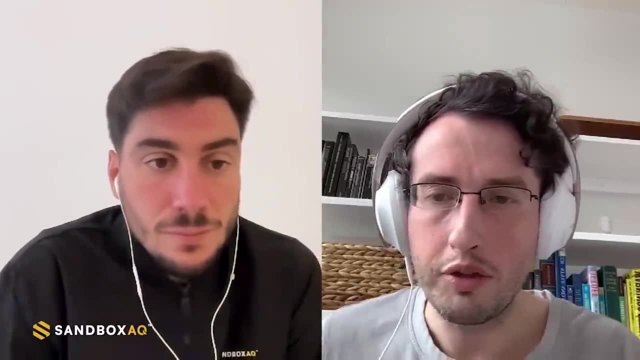 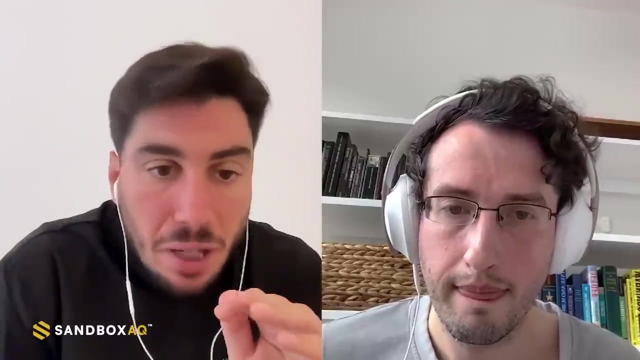 curve based cryptography, which is, you know, based on the hardness of uh, uh, based on similar kinds of hardness problems, and shore in 1994 showed how you could use a quantum computer to break all of that. so basically he said, using quantum computers we will be able to break a virtually any password in the world, something. 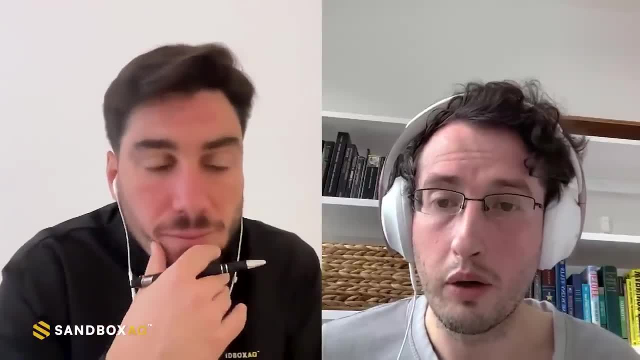 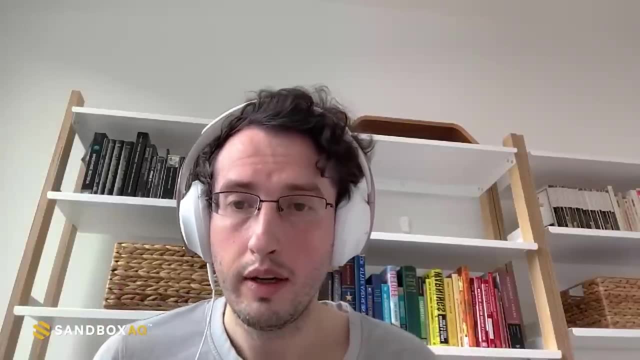 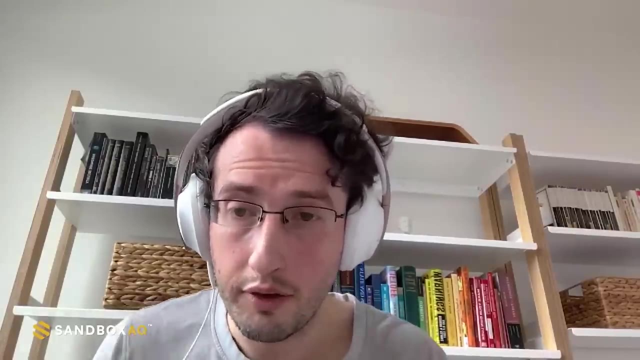 like that, right? yes, exactly exactly, and so that was a big deal. so now quantum computers have- have now, at that point in 1994, been demonstrated. not only is there, are there things that they can do that classical computers apparently can't do, at least not as quickly, but it's very, very. 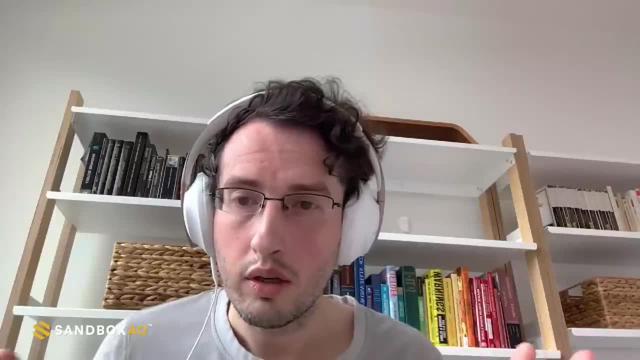 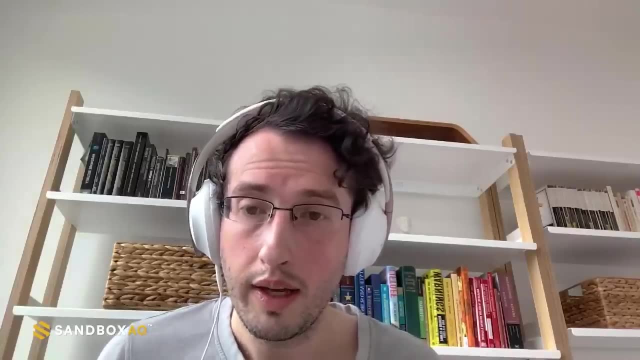 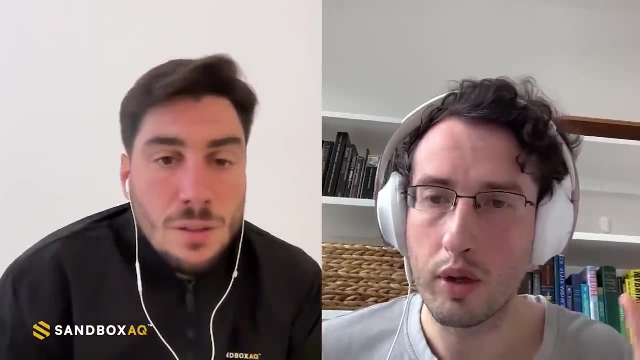 important real world problems, things that would totally change, you know, the. the existence of a quantum computer would totally change the way that we approach cryptography, for example, and this, you know, this was a watershed moment, this little, and at this point it's a sort of a firestorm of. 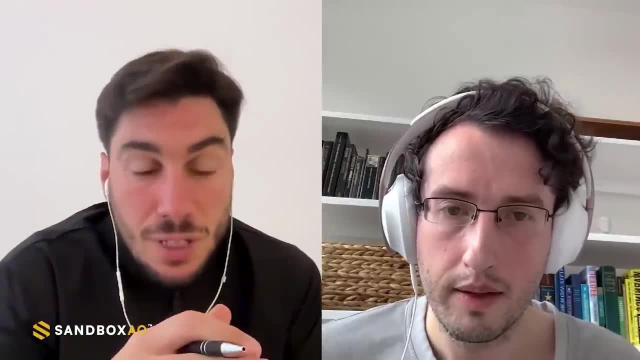 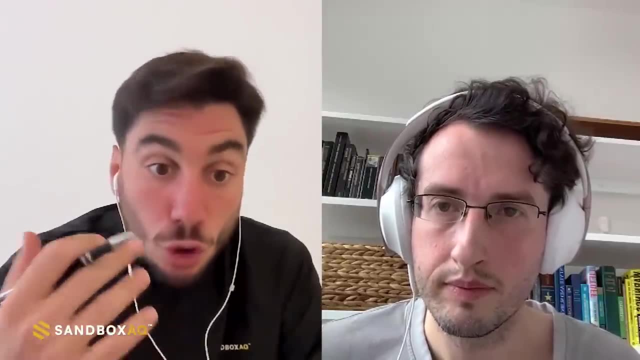 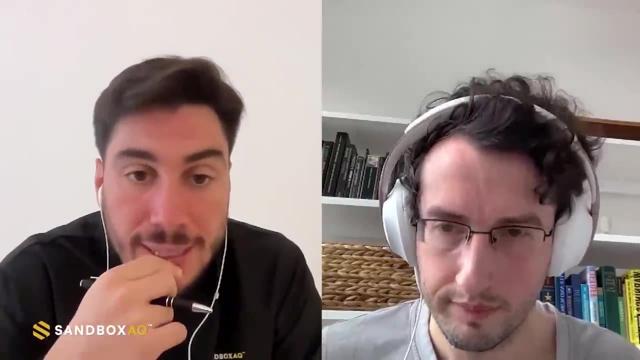 activity from then until today. and then in few years, because this was 1994, four years later, boom, the first working quantum computer is built. some people don't know that we already have quantum computers. uh, this was uh, quote unquote: a small one, two qubits only. but then, a few years ago, at google, 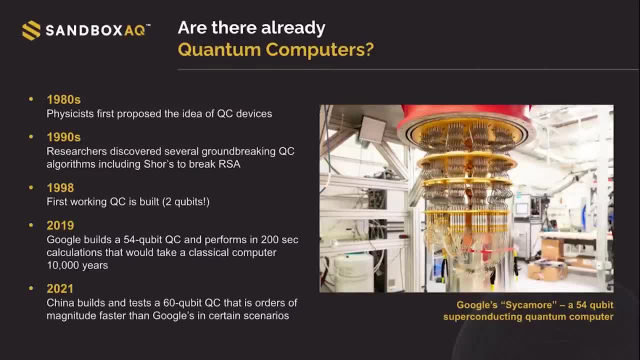 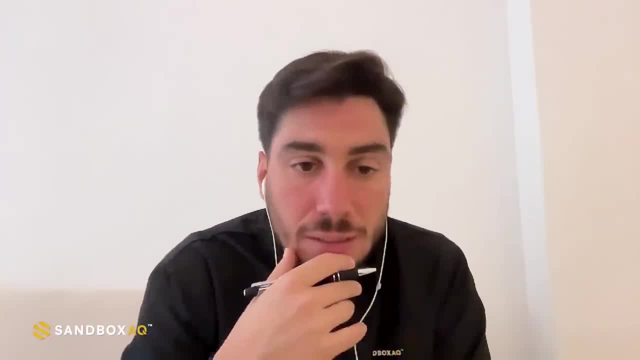 uh, they built a 54 uh qubit quantum computer and which is uh mind-blowing is that uh calculations that our laptops or supercomputers, even uh, will need uh 10 000 years to solve this quantum computer solved it in 200 seconds, so this was also a. 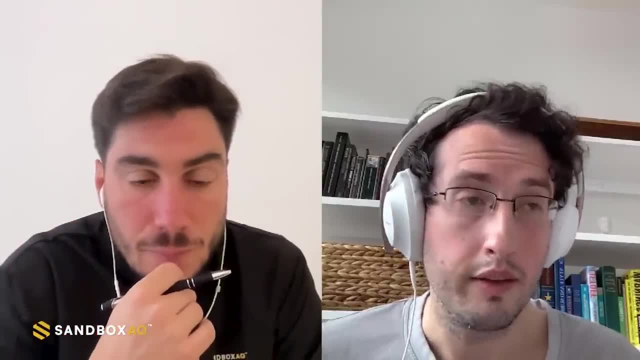 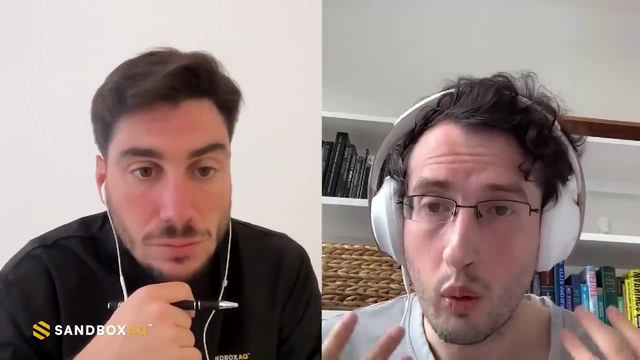 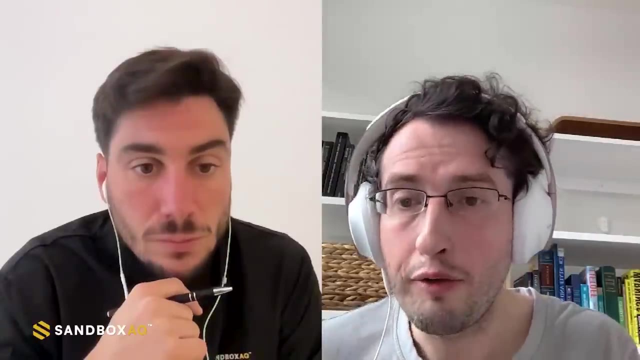 groundbreaking moment. right, that's right, that's right that that, that moment, sometimes people call that moment quantum supremacy, uh, meaning the moment when a quantum computer can start to, like a quantum computer that we've actually built, solves problems that are effectively impossible to solve without using the quantum computer. and we've, you know you can argue about. 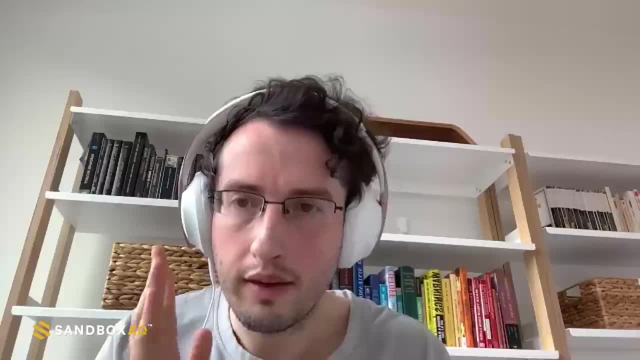 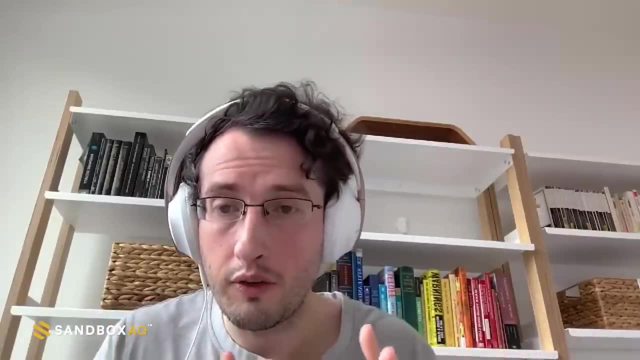 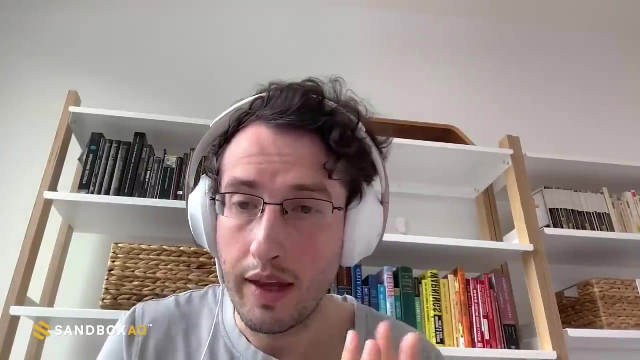 exactly did that? did that literally happen at the time in 2019 when google did? sometimes people argue: but what's what you can't argue with is that that transition into um, the time when an era when quantum computers are actually more powerful in certain senses than any existing classical. 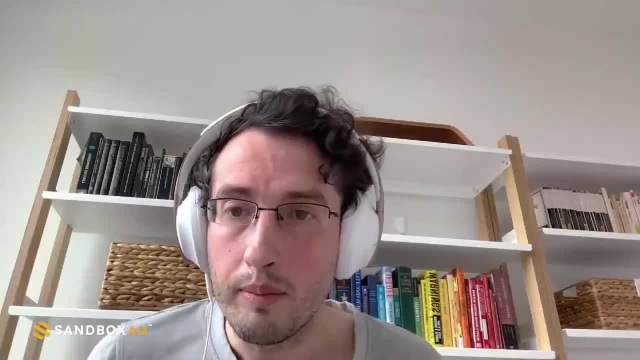 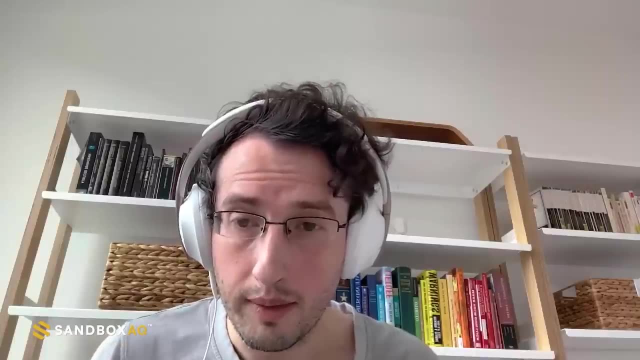 computer. we're transitioning into that era right now. um, it's also important to note, of course, that the the the calculations that they saw that they performed in 2019, they were not factoring numbers. these were not- these were not yet useful calculations. that still is yet to come. 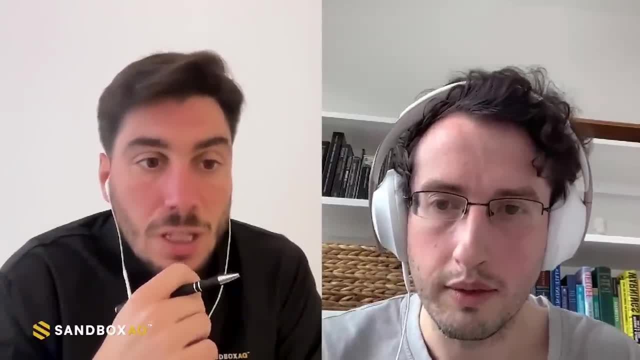 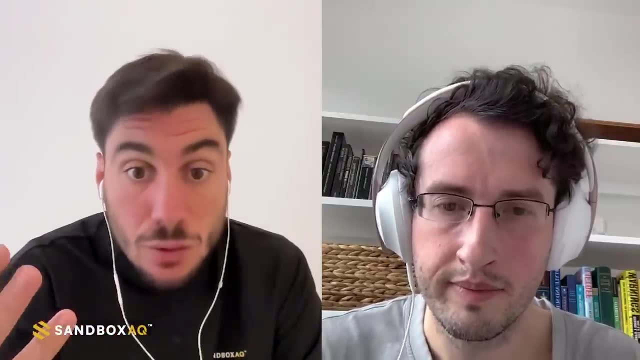 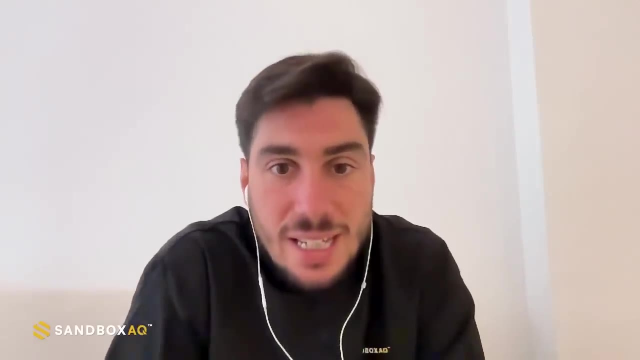 but it's, it's, it shows. it shows that we're progressing. it was a proof of concept, somehow. and then, two years later, china builds an a different quantum computer, with 60 qubit in this case. and then if we uh talk about uh, what is the uh situation now? so researchers what they're looking? 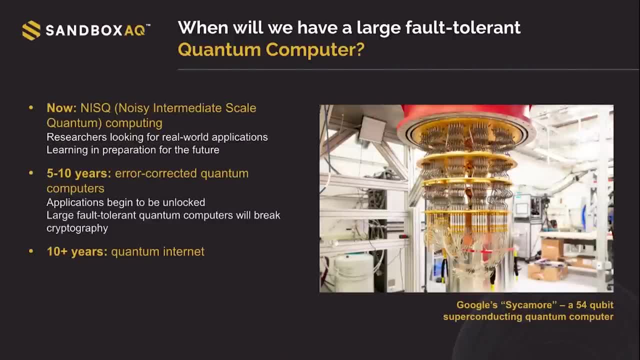 for is a real world application or applications and they trying to find those right like basically not thing going, keeping the exact same size and um, but it says the quantum computers. but by a number of mu facts have stopped in business. there is even awareness that the quantum computers. 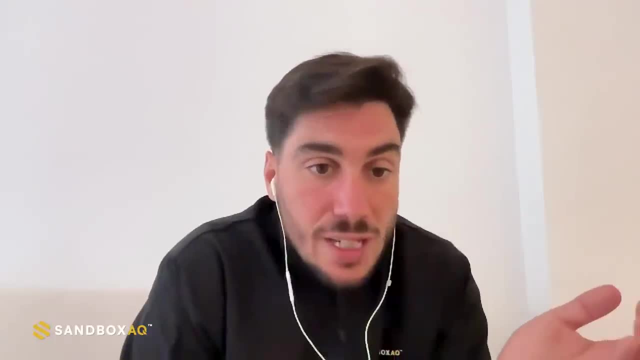 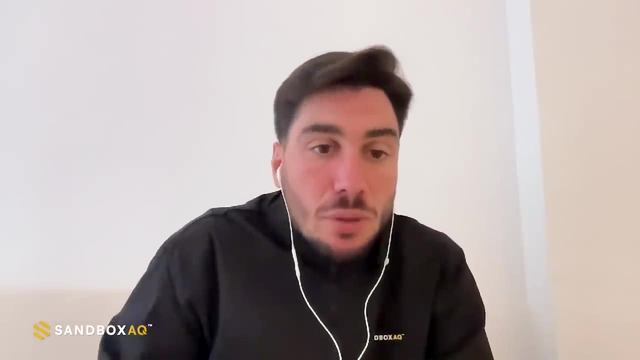 will be continuing to be part of every future and future of quantum computers. it's, it's funny, okay, so, uh, yeah, uh, i was going to ask you something. if, if we want to know, uh, more about quantum computers, perhaps it's a bit like how you got your career in quantum. 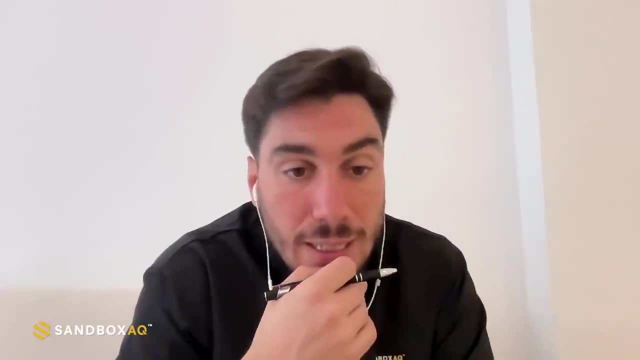 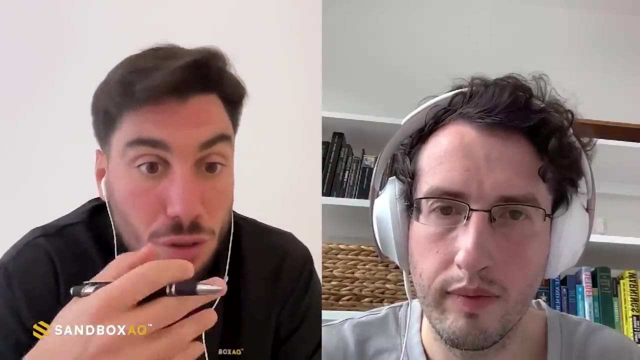 please take a look. where do you think can we get any more, then, for all the opportunities that you may have? um, how do you think can we get more of dignified because, uh, quantum computers- we're here for the error corrected. quantum computers by then, and also we, if we could use them for real useful. 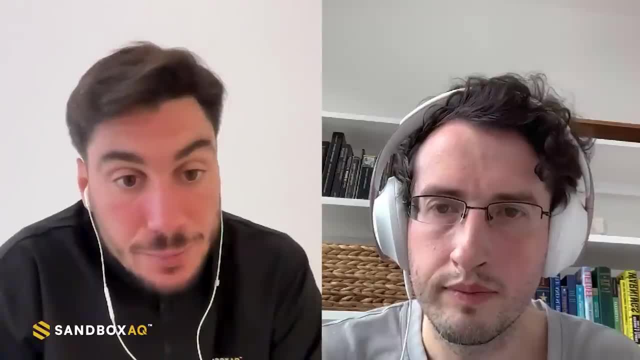 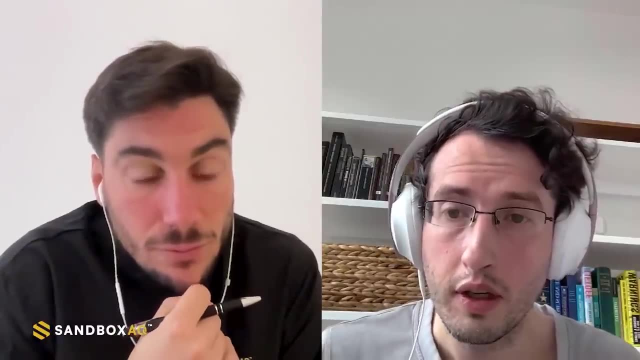 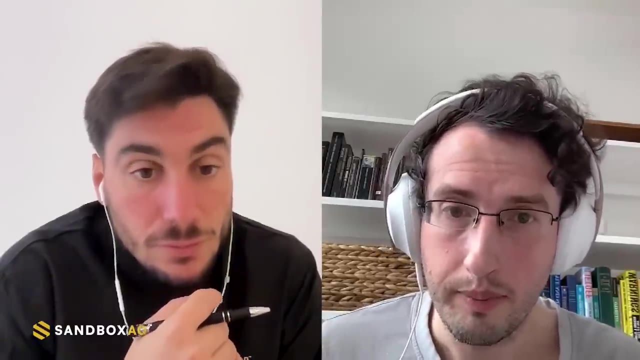 uh, you know real world applications, yeah yeah. so there's, there's sort of two important uh, there's a couple of important points here. first, without error correction, we'll never be able to do something like factor numbers and break rsa, because that's going to require um, it would. 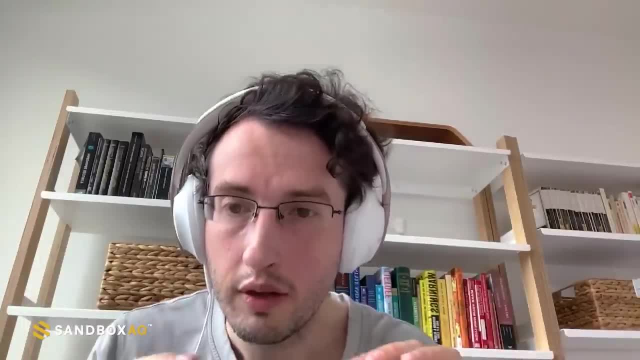 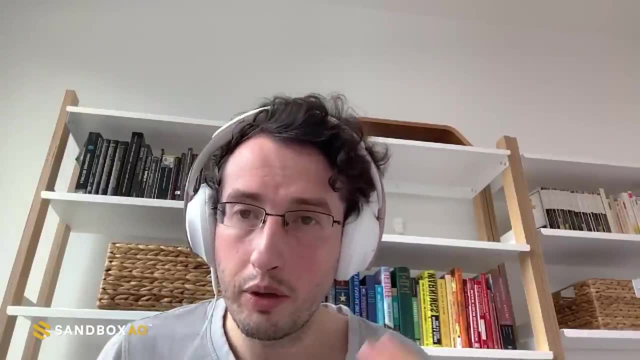 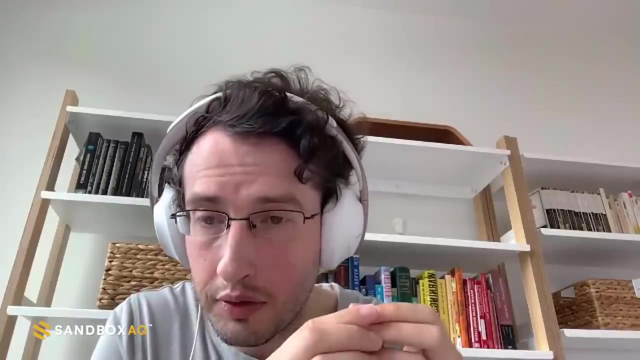 require thousands of perfect, zero noise qubits but, like today, we have 50 or 100 qubits and they're very noisy. so what people do is they use error correction to take a bunch of noisy qubits and distill out an effective what's called logical noiseless qubit, and right now the best, the best. 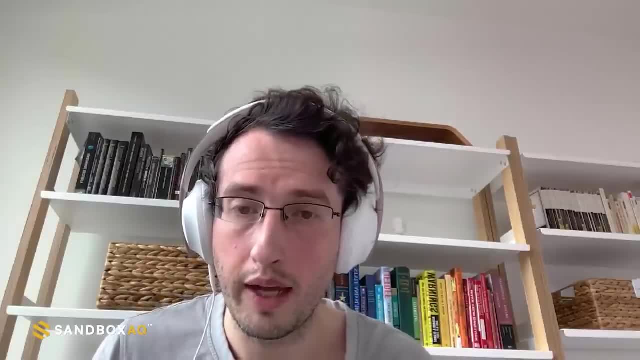 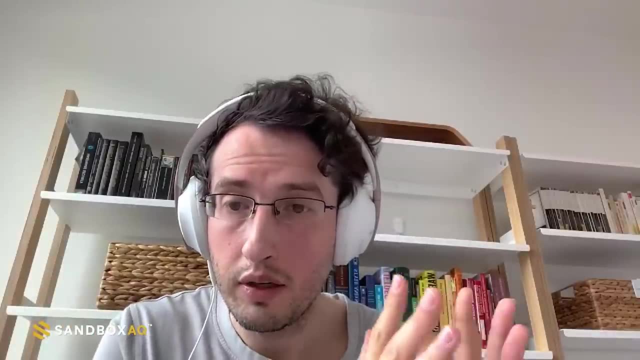 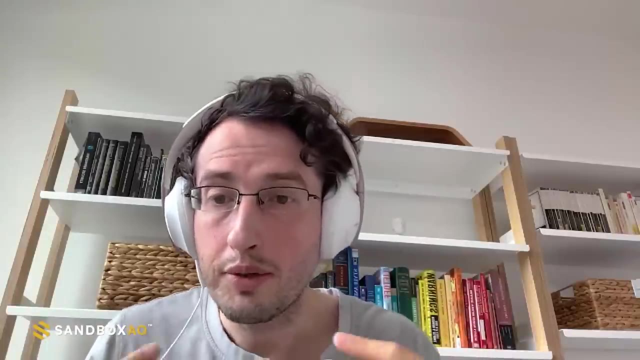 uh, algorithms, or the typical algorithms people talk about, for that require a ratio of a thousand to one. so you need something like a thousand noisy qubits to make a single perfect qubit or a single noiseless qubit that you can then use. and so if you needed thousands of noiseless qubits, well, that translates into millions of noisy qubits. 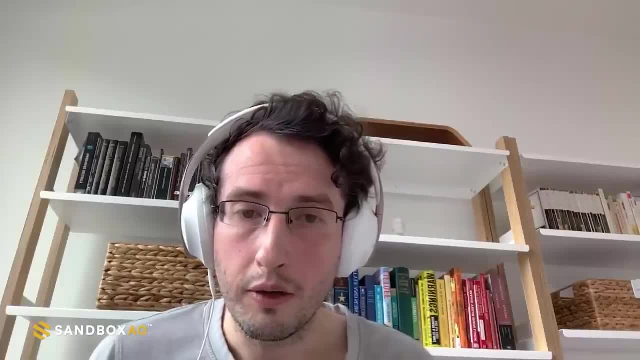 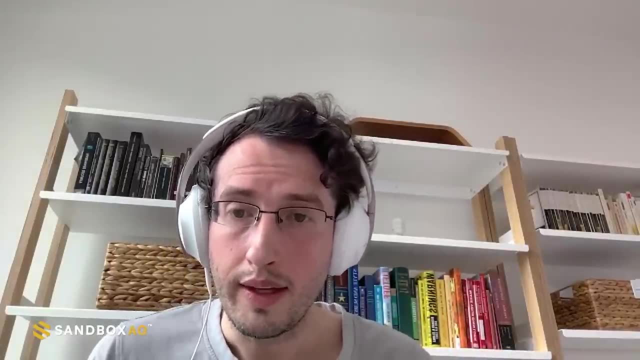 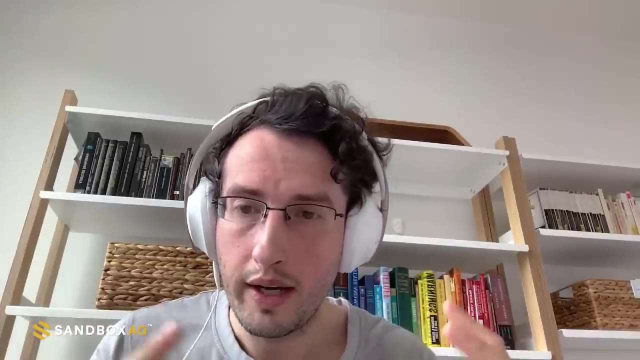 uh, after you take into account this thousand to one ratio. and so what will probably be demonstrated, or what people hope to demonstrate in the not too distant future is, um, taking, you know, hundreds or a thousand, uh, noisy qubits, and demonstrating that they can do this error correction operation right, and that's, that's kind of the next interesting. 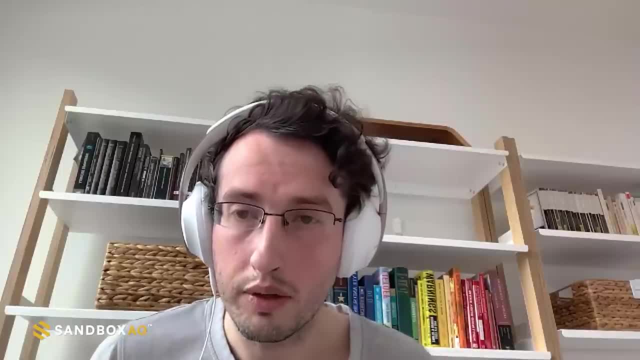 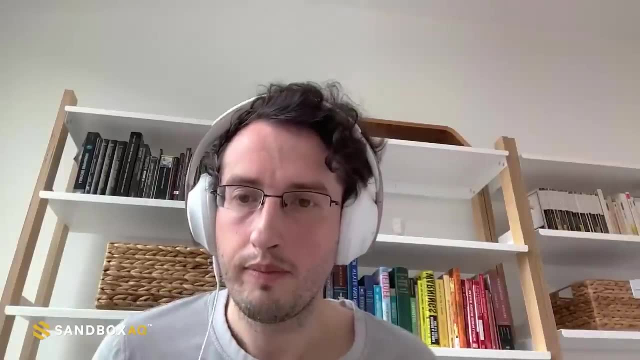 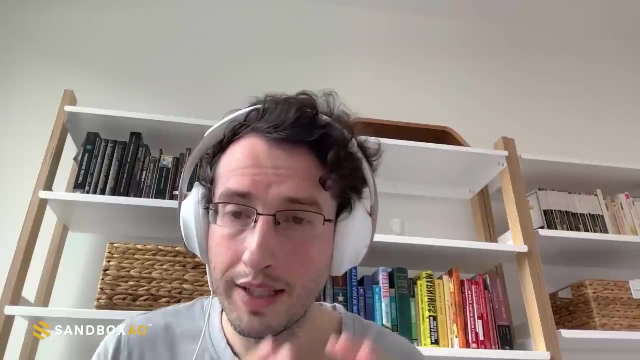 moment, or one of the next interesting moments in the development of the, of the quantum hardware. and then, uh, beyond that, you'd want to say: do that itself a thousand times to get up to the point where you can do a large scale, what's called fault tolerant quantum computation. and that's when 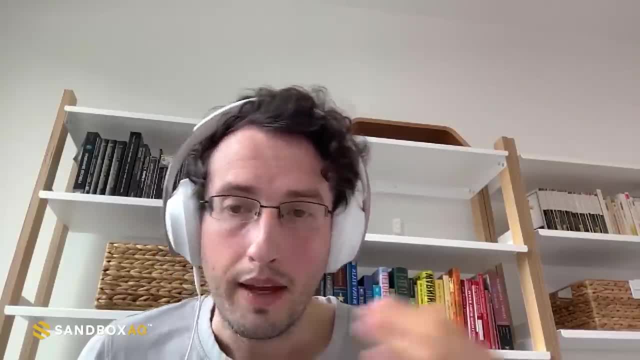 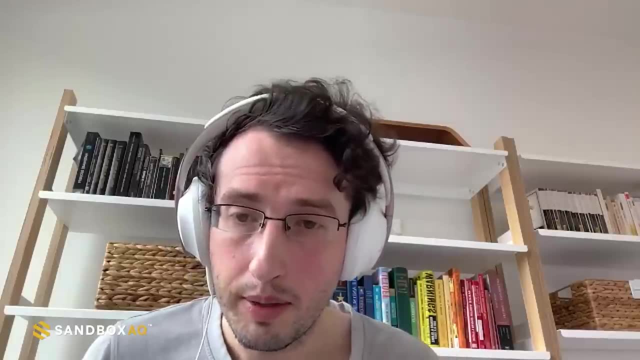 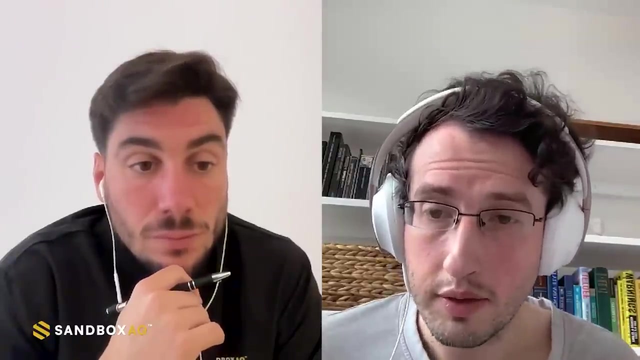 you can do things like run shor's algorithm and yeah, it's really it's. there's a lot of uncertainty that's going to happen. it could be five years, i would say is very optimistic. 10 years is a typical answer that you get when you ask people. but it could be. could be 15 years, but but it is, it is. 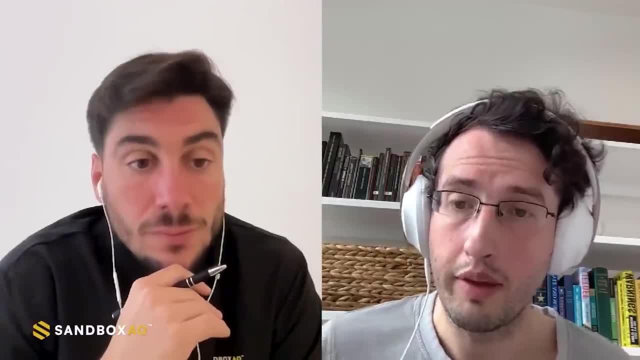 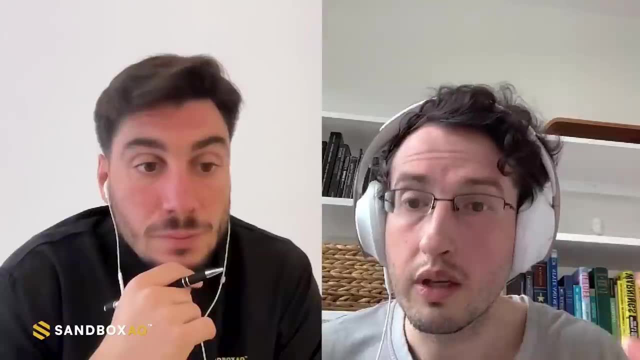 believed. i think at this point that it's really a matter of when rather than if, and it's probably not going to be, you know, 30, 40, 50 years. it's probably somewhere closer to like to this 10 year. 10 year mark got you and then